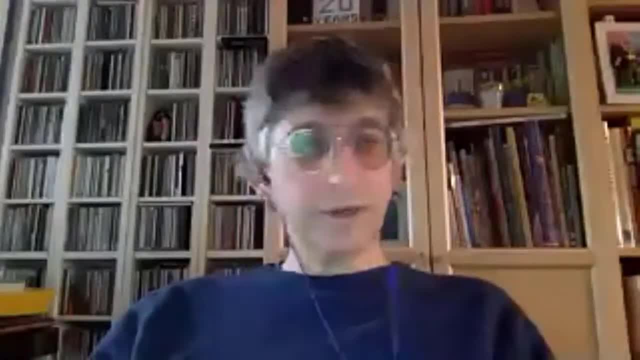 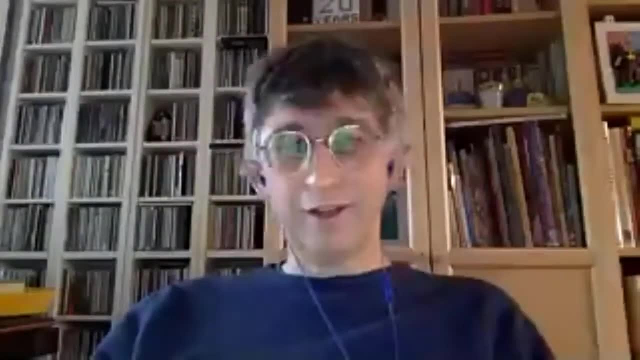 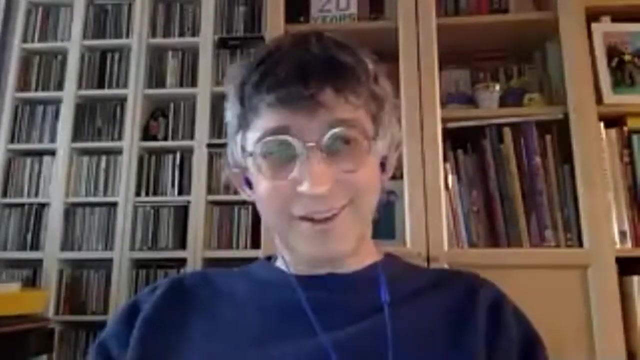 Recording Riley. So I'm extremely pleased to introduce Andrei Marziali, because Andrei stepped in at relatively short notice And he, you know, he told me to remind you that that this is prepared with very little time, But I mean, I can say that because I know it's going to be a great. 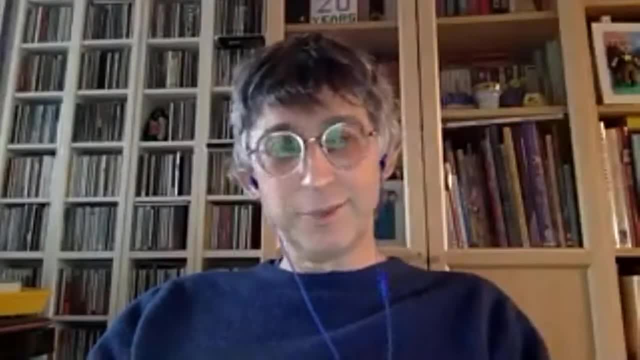 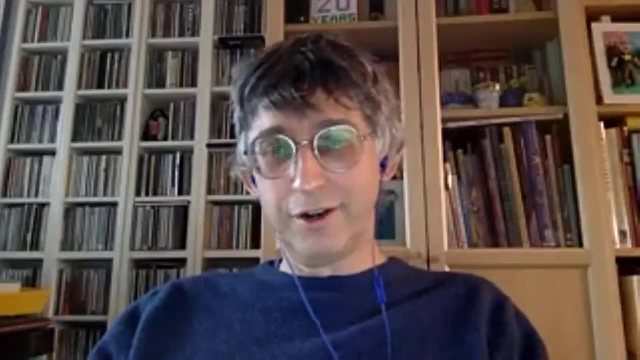 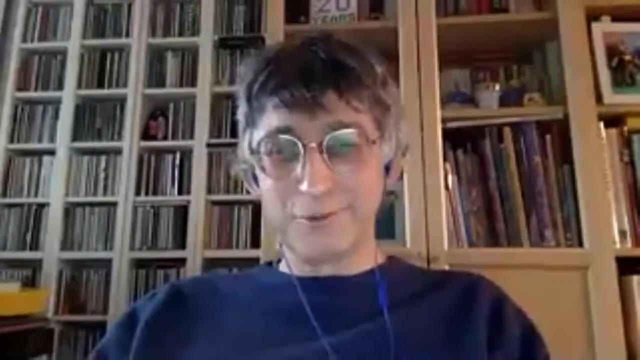 talk. So Andrei has been a longtime member of our department. He's director of the engineering physics program. His research interests are in biophysics and genomics in particular, But his passion, I gather, is racing fast cars. So he sort of put together his hobby and his 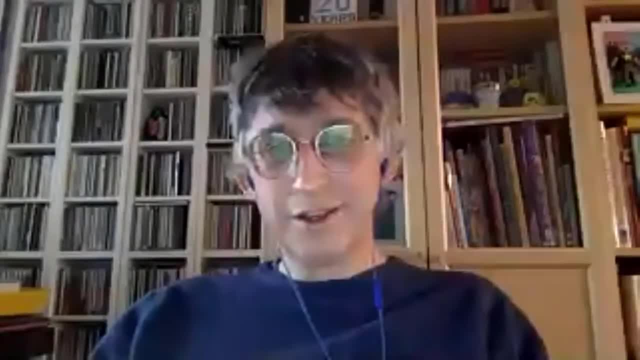 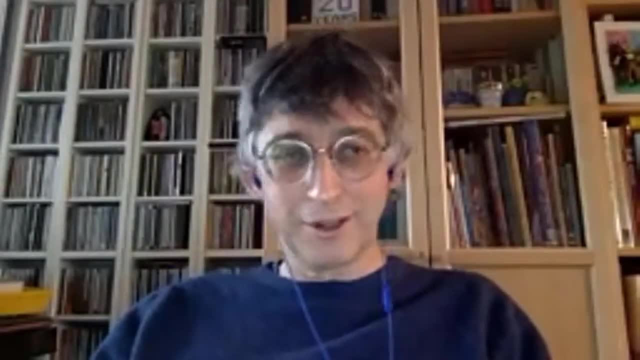 engineering interests and realized that there's a whole bunch of cool things to tell people about the physics of race cars. So that's what he's going to talk to us about today. So, Andrei, take it away. Great, Doug, Thank you, And. 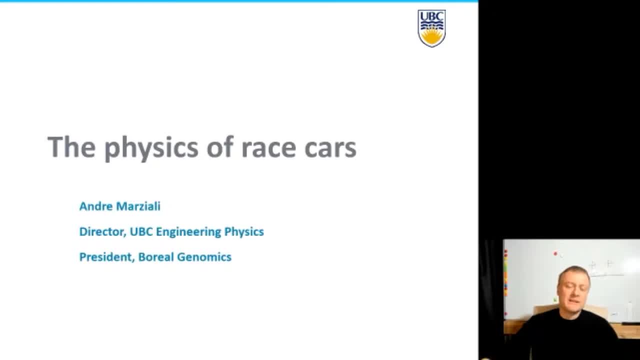 if I run into any trouble with audio and video, please let me know. Yeah, it's a pleasure to come and give this talk. I feel a little sheepish on multiple fronts. One is: this is a talk that's aimed at really beginner race car drivers, So the physics is quite simple. I'm not going to. 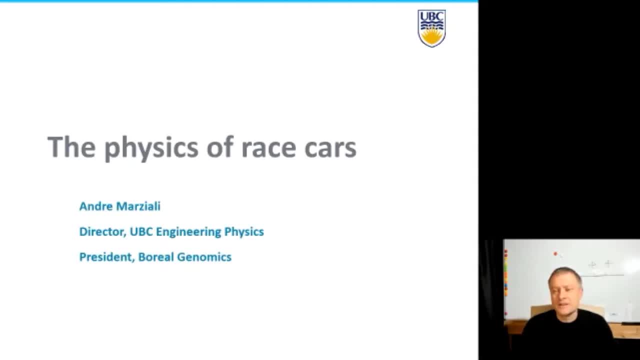 get beyond Newton's laws and some first year physics, although it does lead to some intriguing outcomes. But you know, normally I'd introduce myself with with my academic credentials. I think, for the sake of this talk, I'll have to introduce myself with my 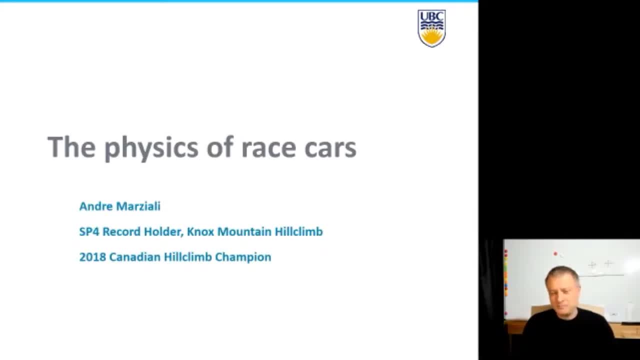 racing credentials as somewhat meager as they are, Although for a brief time I was the the Canadian Hill Climb champion by a feature of winning the Knox Hill Climb, which is now the only Hill Climb in Canada. So I, you know, again sheepish on at the level that I know there's actually at least. 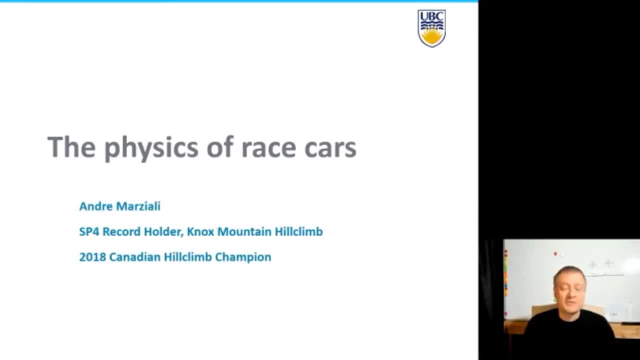 two professional race car drivers in the audience now and at least one professional race engineer. So for those of you that know a lot more about this than I do, please forgive me for oversimplifications at least, if not mistakes. So you know when I first. 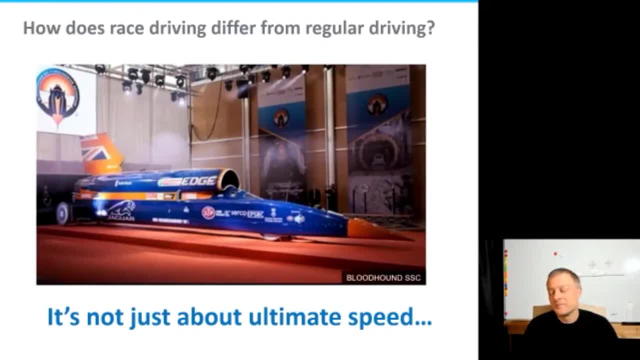 moved into this house with a with a race car in tow, my neighbors quickly came out to sort of ask me: how fast, how fast does it go? To which I shrugged and said I have no idea. I've never had it pointed in a straight line for long enough to know, And I think you know what I hope to do in. 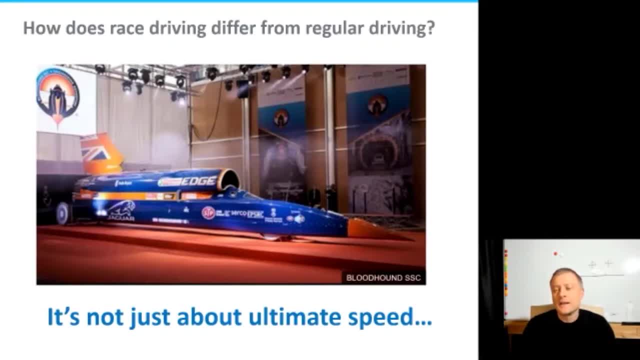 the future is. I hope to be able to tell you what racing really means, And I think that the general concept of racing is not quite what what we think it is. for those of us that race cars, It's not really about speed, I mean counterintuitively. I mean we obviously want to go fast, but there are 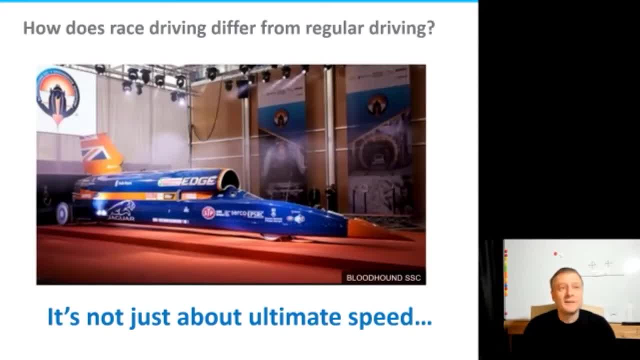 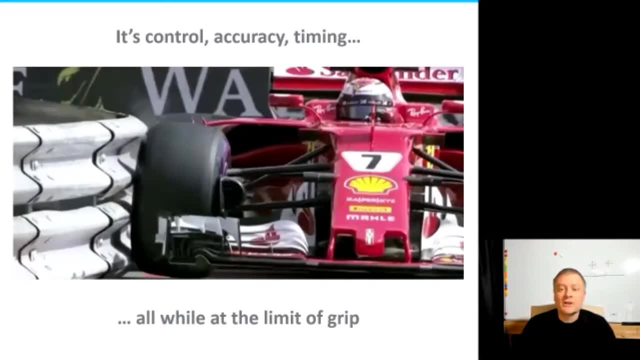 there are sports that are simply around reaching the ultimate speed with a car. Racing is really about the intellectual and physical challenge of being at the absolute limit of what a car can do in terms of grip, while still having incredible levels of control and accuracy over the car and over the timing of things that 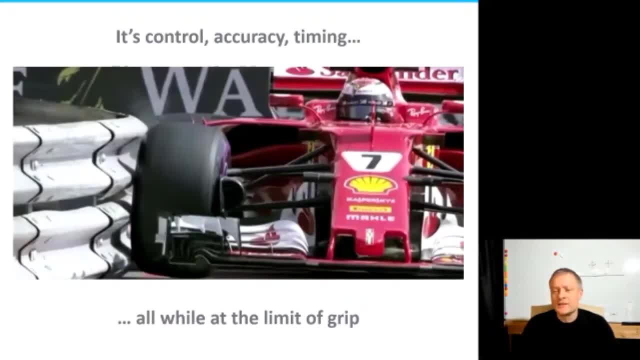 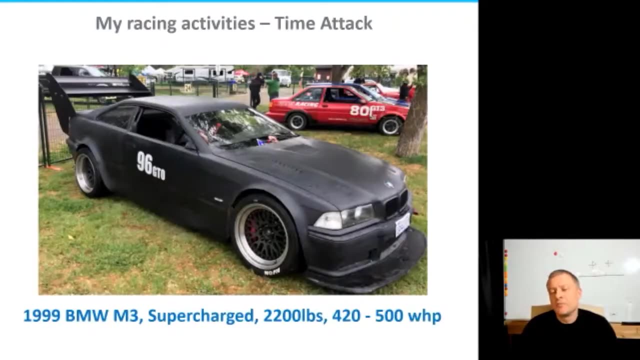 need to happen, And appreciating that on the TV screen is sometimes difficult And I hope maybe I can help you appreciate that through this talk. As a means of a bit of introduction for myself. I'm involved in what's would be known as grassroots racing, So this is a community of 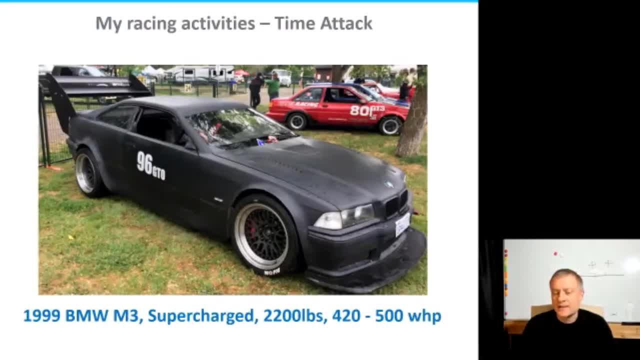 people that tend to modify or build their own cars. This is mine. It's developed off of an E36 M3. But hugely modified. I've chopped the roof off, replaced it in carbon fibre, I've taken about 1,000 pounds out of the car and increased its horsepower to somewhere near 400 to 500 horsepower. 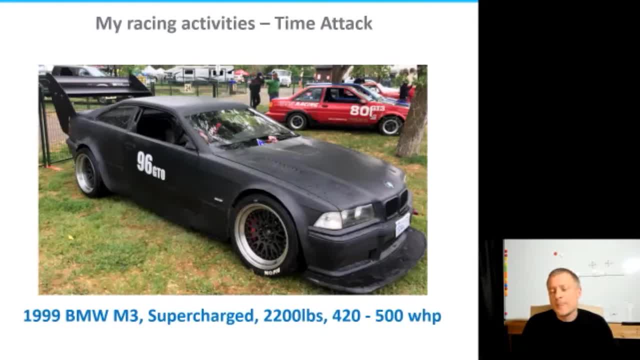 somewhere in there. The type of racing I do is what we call time attack. So it's really trying to hit the fastest possible lap times on a closed circuit, obviously, and without necessarily having or without having to pass other drivers necessarily. So I'll show you a brief glimpse of the Knox Mountain Hill Climb. 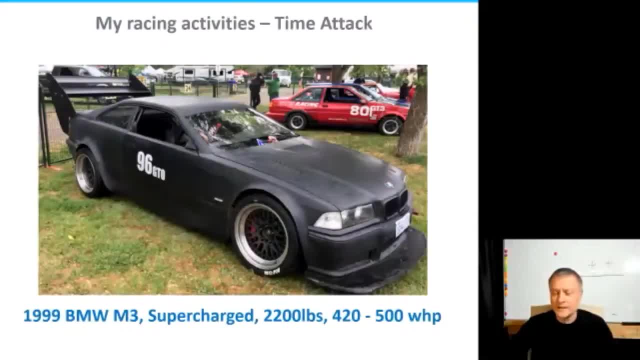 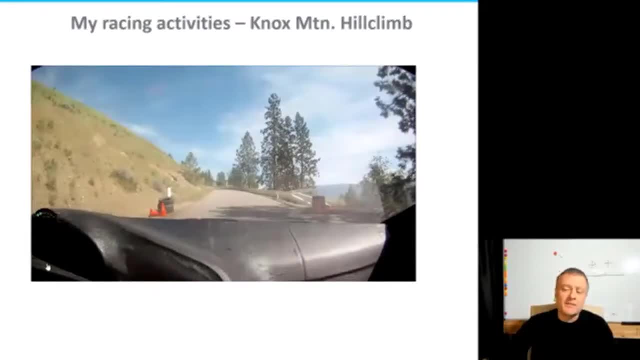 which is my favourite event of the year, And unfortunately it just got cancelled for this year again. But when we used to run it, it would look something like this: You're driving at very high speeds, upwards of 180 kilometres an hour, but on a paved mountain road where there's trees. 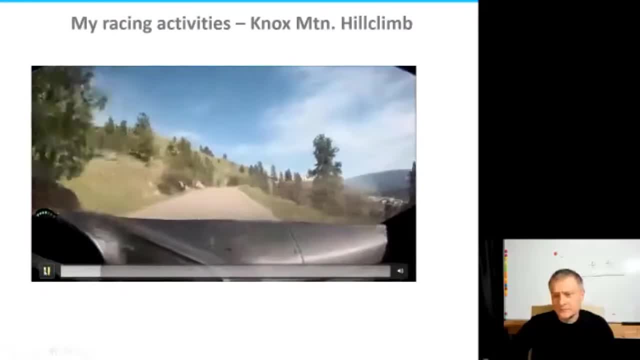 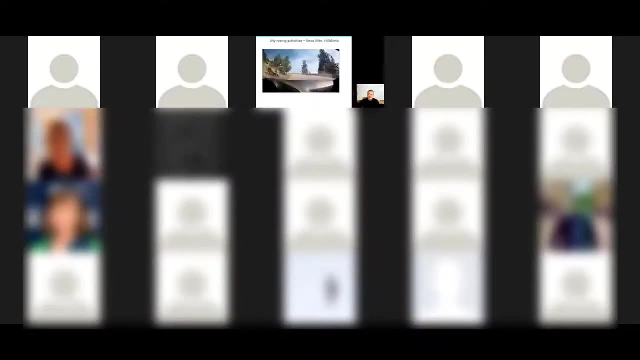 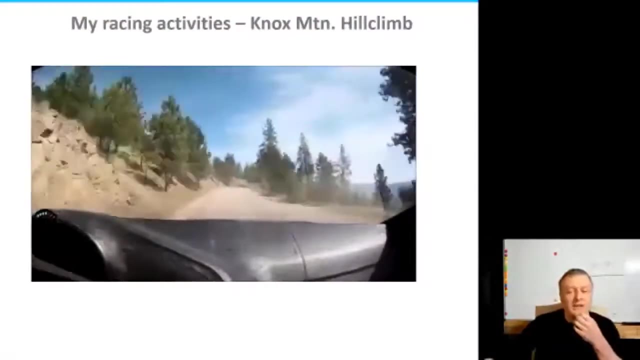 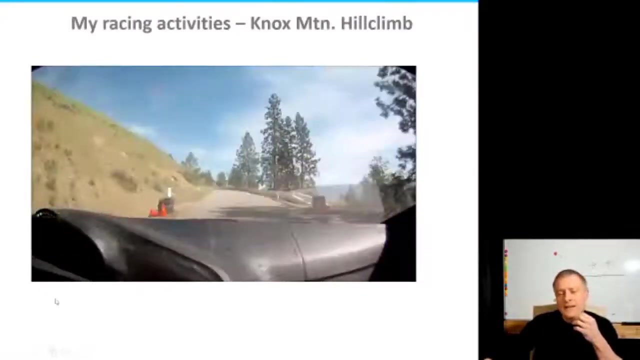 and cliffs and so forth. So psychologically quite a challenging event. Making mistakes on a course like this doesn't lead to run off into the grass or gravel. It can lead to making contact with a cement wall or going over the edge of the mountain or something to that. 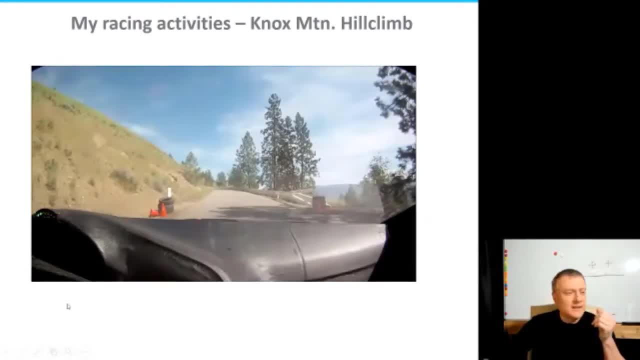 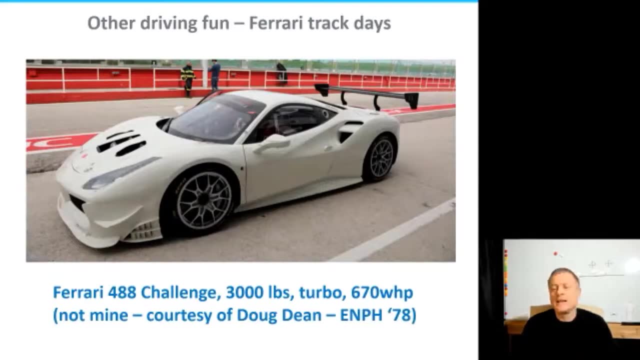 effect. I've done one of those two things twice. So I also have the incredible good fortune of a friend and colleague, ex-alum from EnschVis of 1978, who lives in Switzerland and has had a wonderful career and owns a number of Ferrari cars. 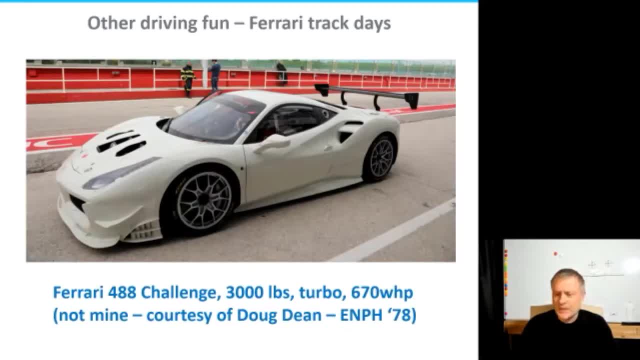 including two or three Challenge cars, And he's been kind enough to invite me to Europe to race them year after year, And so I've had the pleasure of driving some cars that I've not built in my garage and then actually performed properly, And with those, 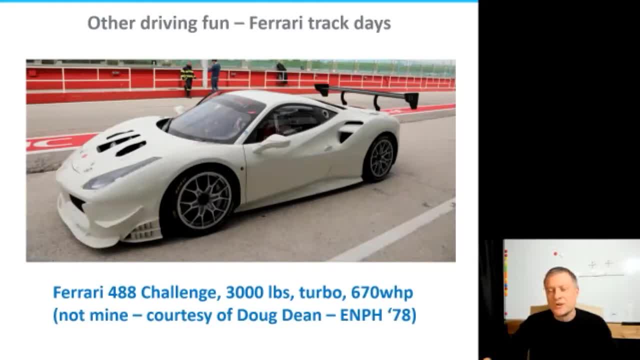 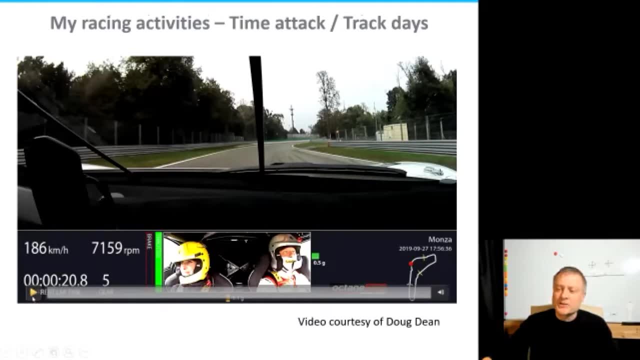 I've had the pleasure of racing on circuits where you can corner, And here this is an example, at Monza. This is Corva Grande at Monza, where I've had the simultaneous pleasure of cornering a car at over 200 kilometres an hour, at the limit of grip, while 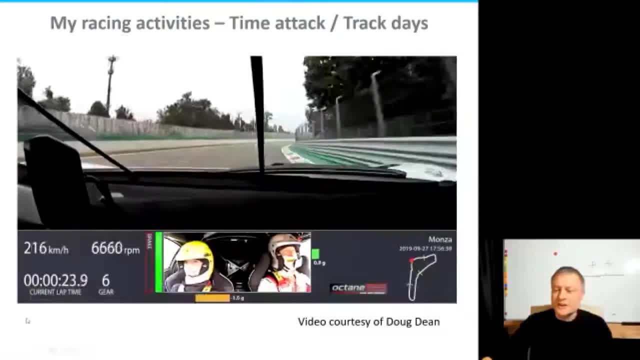 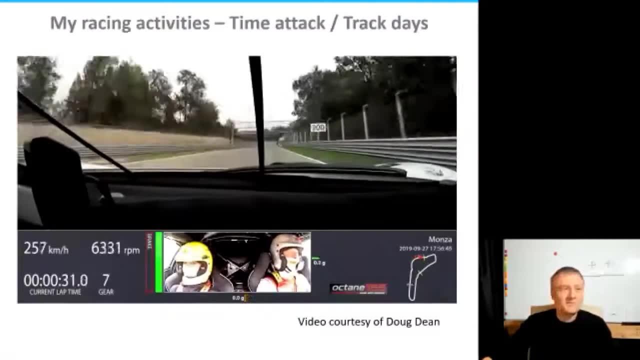 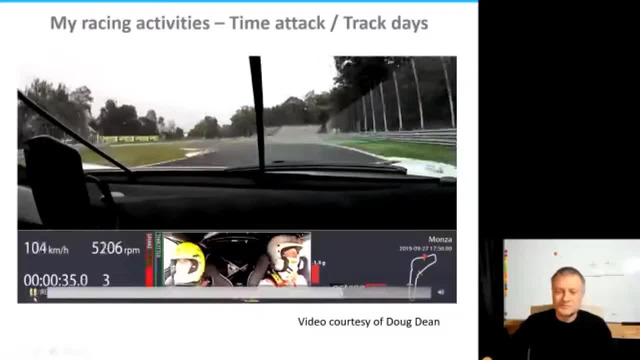 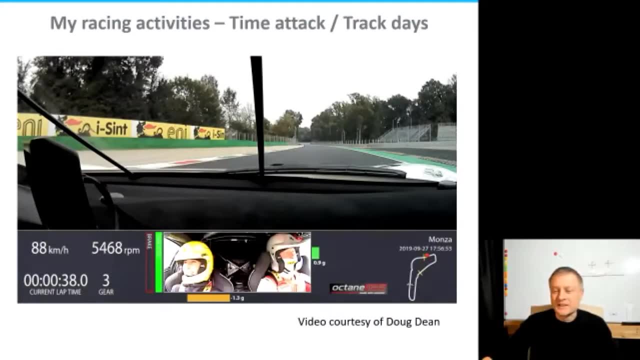 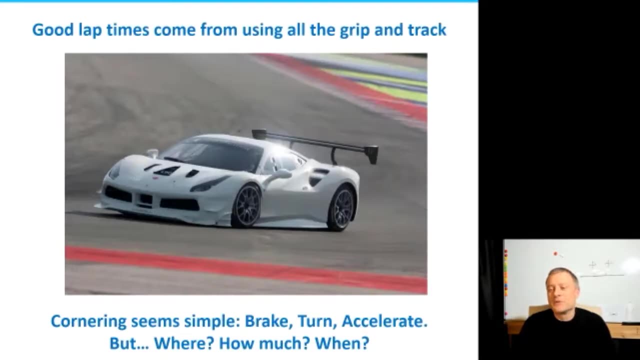 So thank you so much to Doug for that opportunity. So what are we trying to achieve as race drivers, whether amateur or professional, I think we all want the same thing, which is the shortest possible lap time. 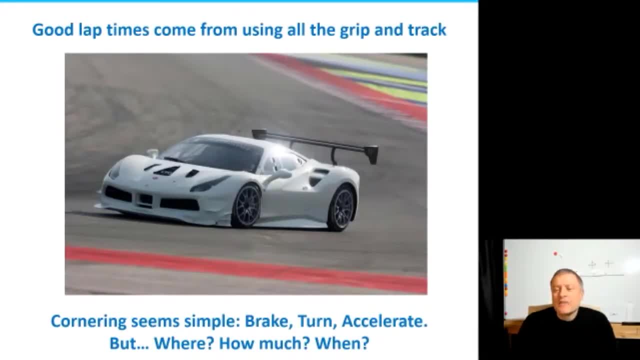 Now, as drivers on the straights of a track, there's not much that we can do short of keeping the pedal all the way to the floor and counting the time to the next corner. It's really in the corners that all the time is made up And, you know, at first blush cornering might seem quite 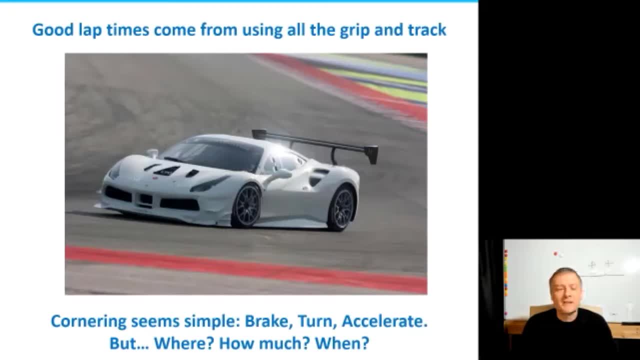 simple. you know you have to brake before the corner, you turn and you accelerate. But the challenge of racing is really, you know how do you do that, How much, At what point, Where do you position the car on the track And controlling the car through that process. So you know. 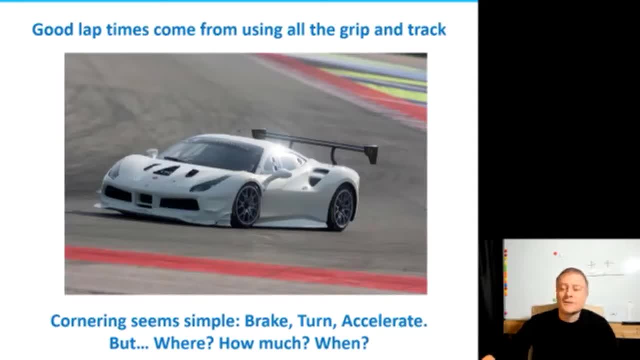 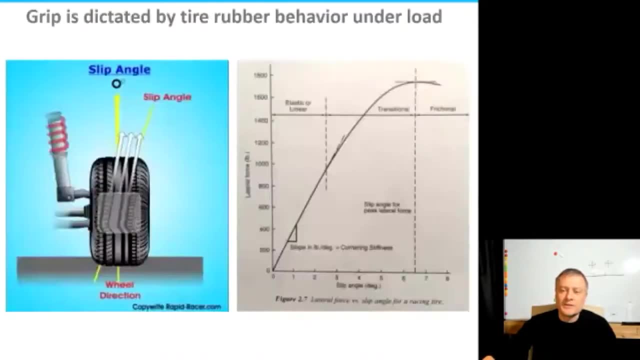 and, ideally, staying at the limit of grip all the time. Okay, so that's really the challenge for race drivers: balancing all the inputs that one has to maintain the car at the grip limit. Now, if we're going to talk about the grip limit, obviously we have to talk about tires, So this: 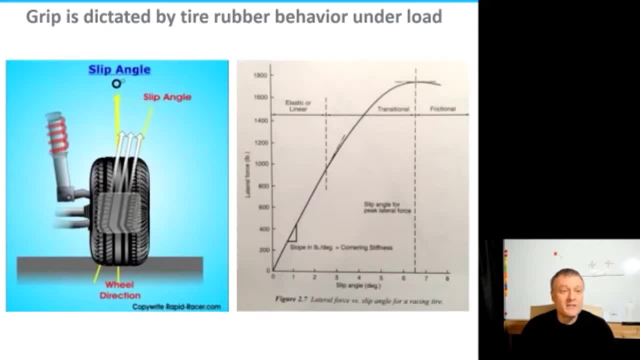 is the most important and most complex part of a race car is actually the tires and how the tires contact the ground, And a lot of the work that we do when we set up or modify cars is making subtle changes to this. Now tires, obviously. 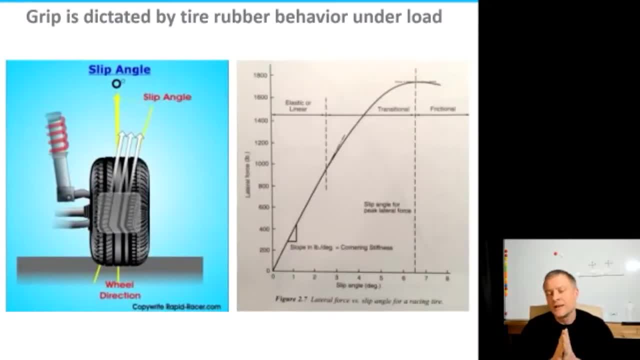 they're rubber, they're filled with compressed air And, you know, they create an elastic surface in contact with the ground. So this is kind of a cool graphic showing a tire rolling in this direction right, or at least pointed in the direction of the big yellow arrow. And what the 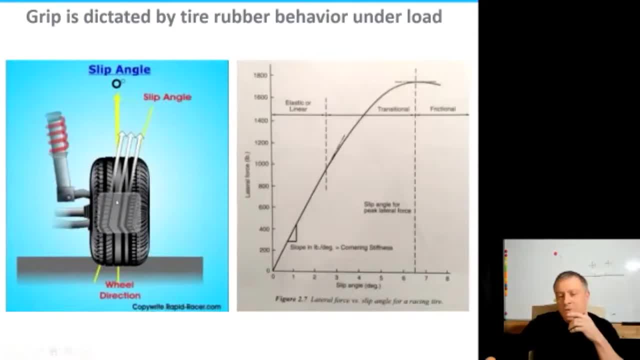 graphic is showing you in this square little window is what the contact patch of the tire with the ground would look like. So you know, if you're going to be driving a car you're going to have to be very careful with the direction of the tire And what that looks like during cornering. 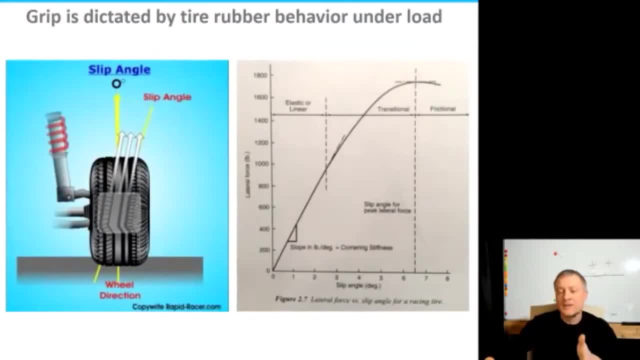 So if the tire is upright and rolling straight and pointed in the same direction as direction of the car, there are no lateral forces on the tire. But as you start to turn the steering wheel to orient the tire differently from the direction that the car is moving in, then this generates what's known. 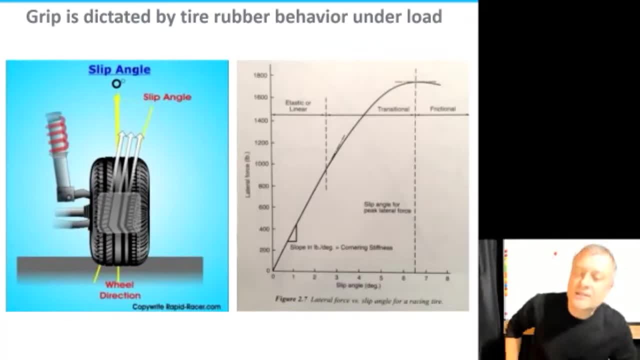 as a slip angle, And it's probably poorly named because a small slip angle. there's no slip involved. really, what's happening is the rubber as it rotates around the tire and comes into contact with the ground. In a slip angle, the rubberなんです back and stays in contact with the께 direction. 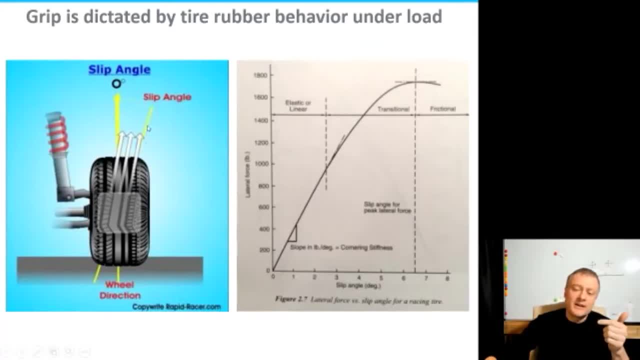 In the frame of the tire. That rubber is being pushed sideways by the road. that is obviously traveling in an angle with the direction of the tire. So you can see in the graphic. you see the treadmill bending And then, as the treadmill comes out of contact with the road, it snaps back. 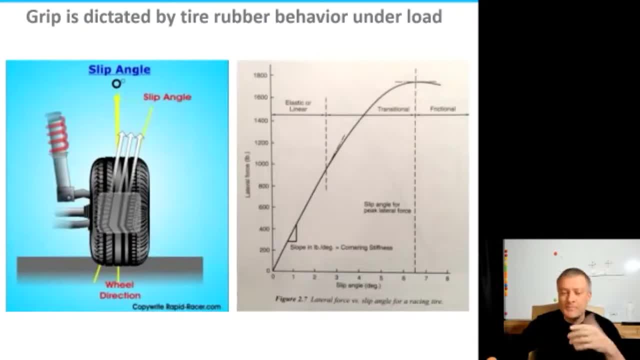 and keeps rotating around the tire 58. Now that bending obviously creates a reaction force from the elasticity of the tire right. So this is a hook sloth in And that's what creates ället, creates a cornering force. so that's how we get transverse force on a tire that will help the car. 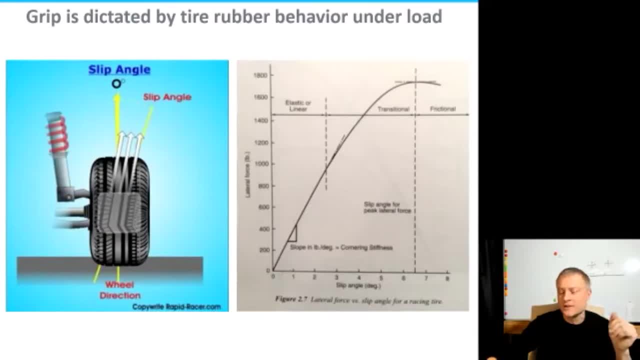 uh, turn into a corner and will provide the centripetal acceleration needed to stay in a corner. now, the more you increase the slip angle, the higher the force increases to a point okay. so for small slip angles this is really an elastic effect, which is why, when we drive around, 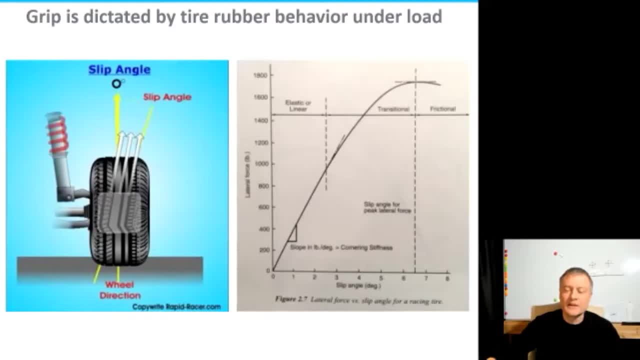 on the street, our tires can last several years. okay, so on the street you're operating in this regime of a tire: small slip angles, um you know, and relatively small amounts of lateral force. that's not where race drivers operate. race drivers operate up here. so as you keep increasing the slip angle, eventually the tire deforms as much as it possibly. 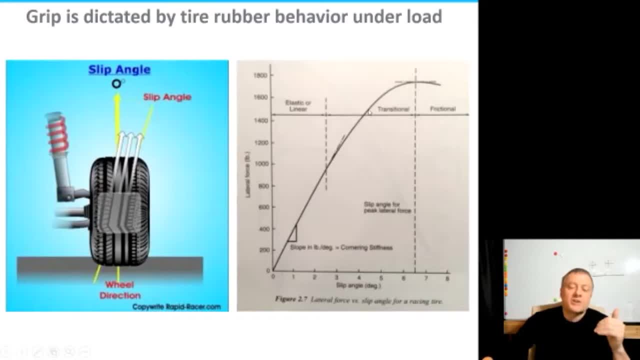 can, and you eventually transition to where you are actually, uh, sliding somewhat and the rubber is is being either scraped off or literally melted and and flowed across the the width of the tire and, uh, you start to operate in a regime that's largely frictional right. so now we can start to 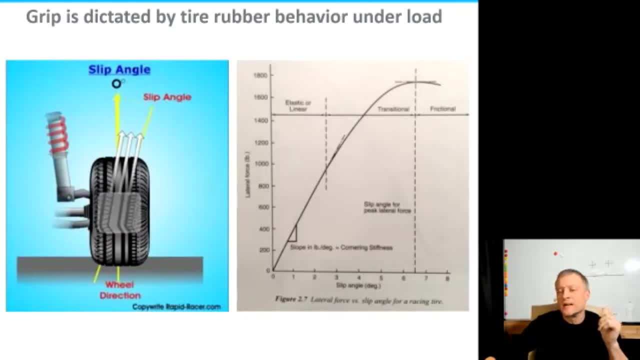 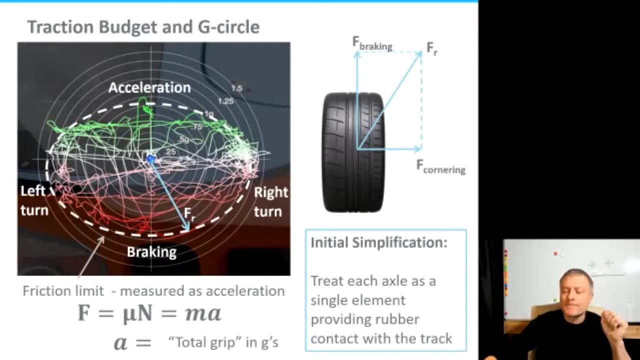 talk about a friction coefficient, uh, between the load on the tire and uh. you know there's a normal force and uh and the cornering force that can provide now that friction coefficient when we get to the friction limit, um of the tire behavior. actually, let me go back and say 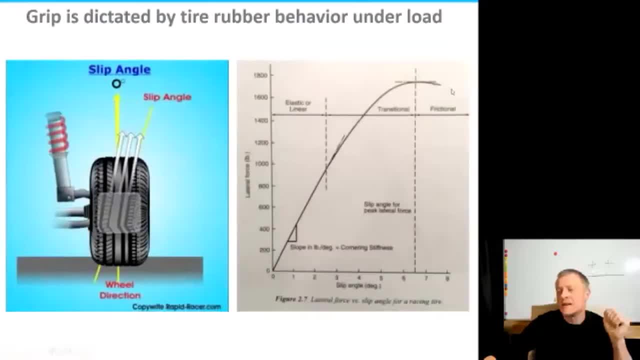 something else, because this curve doesn't go very far, but if you were to keep plotting at a higher and higher slip angle, the cornering force decreases rapidly. and this is one of the real challenges of driving fast is trying to stay at the peak of this curve, because if you, if you, overshoot it, 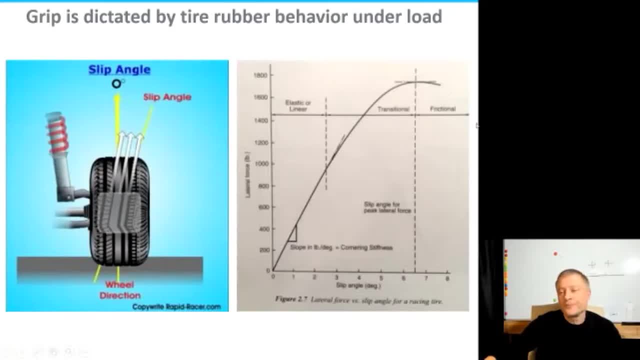 uh, you will rapidly lose grip, um, and of course, if you undershoot it, you're not going as fast as you could. okay. so one of the challenges: really estimating- and a little bit it's got to be by the seat of your pants and intuition sort of what the right speed of the car is in the turn. 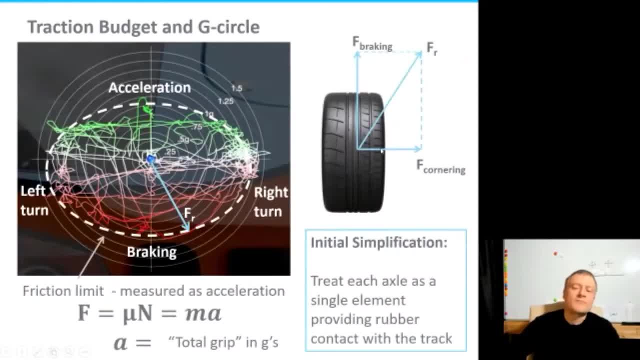 to be right at the peak of this curve. now, on top of that, you know, this friction coefficient is relatively isotropic in different directions in the tire, meaning there's a similar um slip angle versus uh force curve. uh that one would apply under braking or or under acceleration, where power is being applied to the wheels right. in that case, 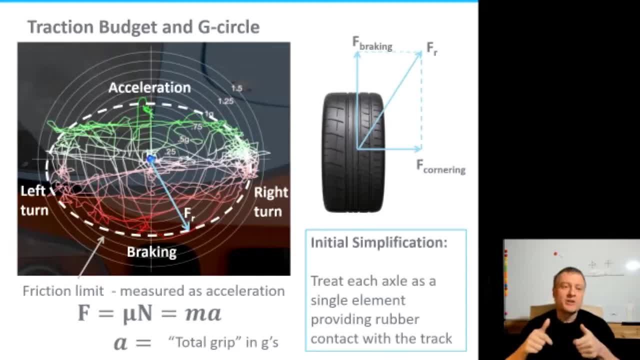 slip angle is: is the number of degrees of over rotation of the tire per second. uh, when you're, when you're applying power and you're trying to spin the wheel faster than than the uh, than the speed of the car at that point, or the, you know the rotation the wheel would have at that speed and, of course, under braking. 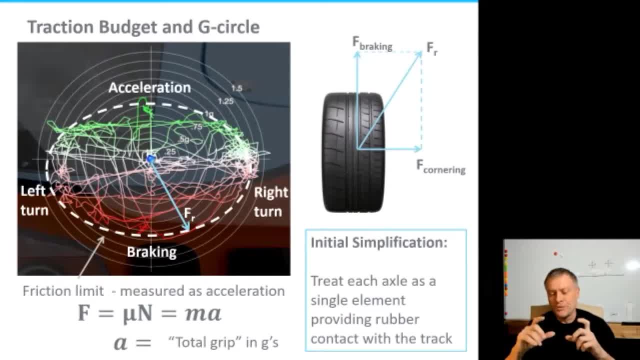 similarly, there's a there's an under rotation of the tire where, by applying the brakes, you're trying to force the wheel to rotate more slowly than it normally would, and that also creates a form of slip, slip angle, and that creates longitudinal forces um the curves, for those 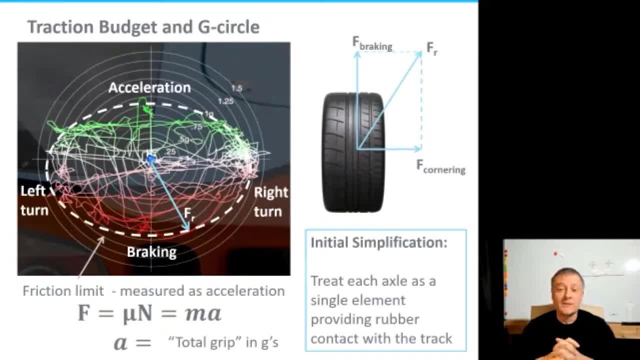 look very similar and, uh interesting the the point where the transition from elastic to frictional are also relatively similar and, like i said, are a form of friction coefficient and if you were to draw, you know, really simplifying. i think this is the first of many, uh, simplifications are going to. 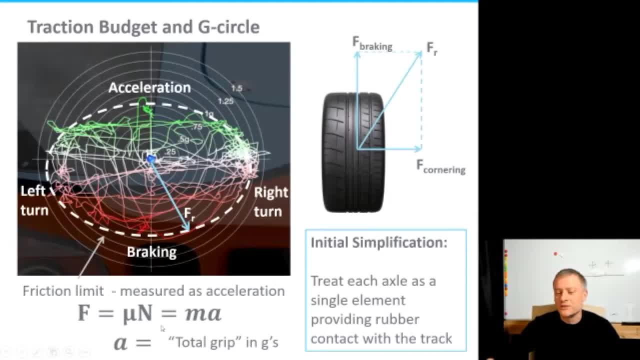 make today that f equals mu? n, right? so you have normal friction formula from first year. that gives you a potential acceleration, either longitudinally or laterally, of a that um, all of us in the racing community really uh speak about in terms of g. so we normalize to, to gravity, uh, which again means 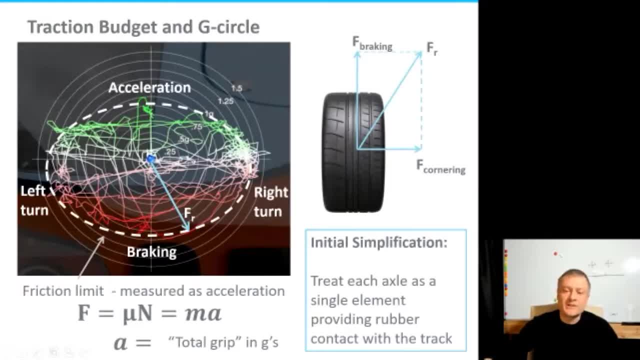 that the acceleration as we talk about is actually almost a friction coefficient in a sense. now, if we look at the performance of a car- and let's say a car is a lot of gas, uh, and we look at that in terms of car performance on what's known as a g circle, where you have maximum braking deceleration. 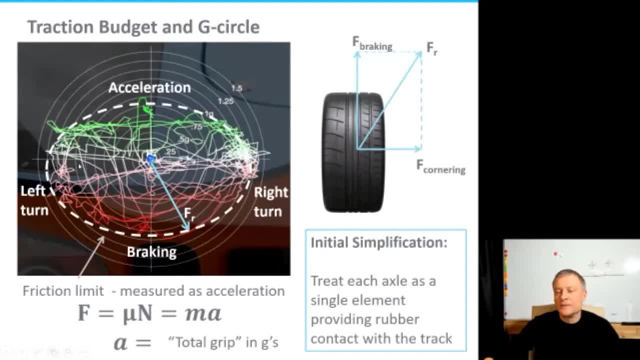 is down here. maximum power acceleration here, this is often engine limited, of course. uh, braking is not. and then cornering left and right. what happens is that at any point, as you're, as you're racing, you're going to be on, ideally, on the edges of that performance envelope and you have to be trading off. 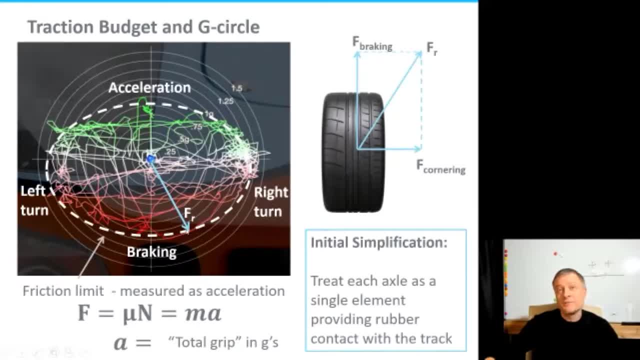 under braking, for example, with the amount of frictional force you ask of them under uh for cornering, because obviously, if you ask your tire for peak cornering grip and peak braking grip, the resultant vector is going to be one that exceeds the maximum uh, you know, allowed friction. 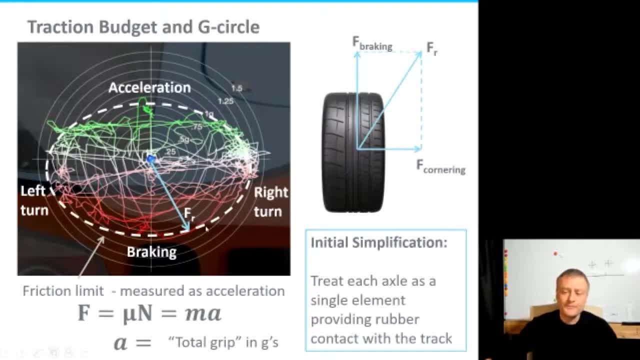 vector for that tire compound in those conditions. now, uh, one thing, i will say two, two quick asides here. one is: uh, for the beginning of this talk, i'm going to treat, um, the car as having two grip elements, the front axle and the rear axle. we're not going to split those axles yet. i'll do that. 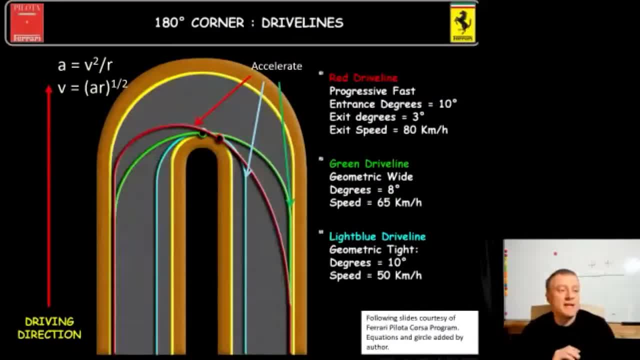 later. um, and the other side i'm going to say is that we need to quickly talk about, uh, racing lines and drive lines, so just to give you a sense of what happens, uh, and the trade-offs that need to be made in the corner. so let's look at a hairpin, and these slides are courtesy of the ferrari. 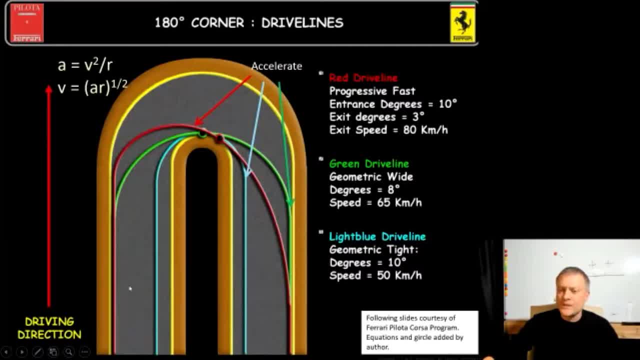 driver training program. again on a road car, if you approach this hairpin, first of all you would coast in and then you turn kind of in the middle of the road, um, or on the right hand side, ideally. uh, not what you do in a race car. uh, of course, if your limitation is fundamentally, grip right, and that grip uh gives. 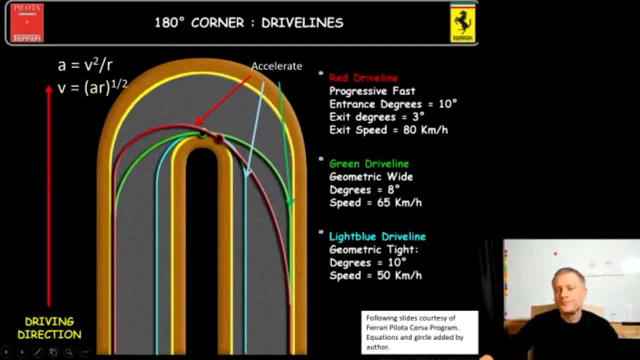 you a fundamental limit in centripetal acceleration in a corner, then it's clear that your maximum velocity to that corner will be, uh, with the maximum possible radius. it goes around the square root of the radius, so the blue line, of course, would follow a very tight radius of that. 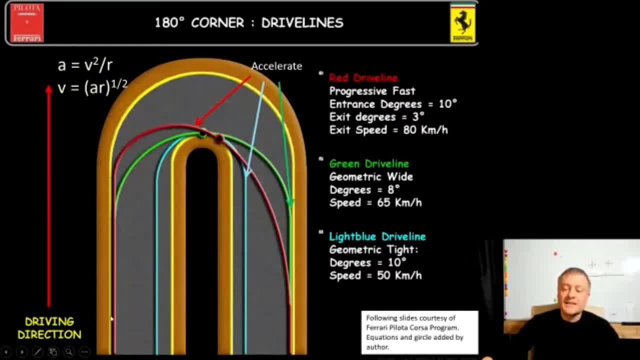 turn, so that's not your high speed line. uh, the high speed line perhaps would be to go around the very outside of the turn, where the radius is the biggest. um, but of course, uh, you're traveling a much greater distance. now, imagine just taking that line and moving it closer to where you're. 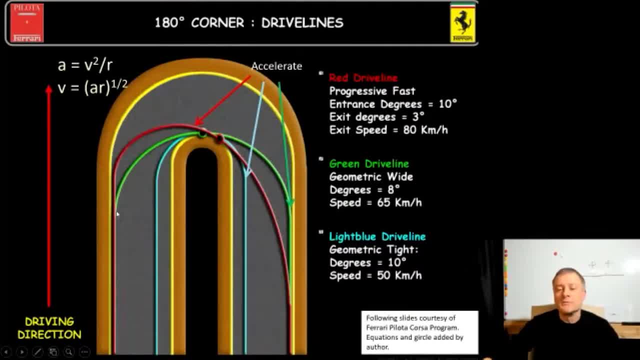 coming from down the track and you get what is sort of the geometric optimum racing line, which is this green line right. so you start at the very, very outer edge of the track and you turn into what's called the apex point right, and then back to the very outer edge of. 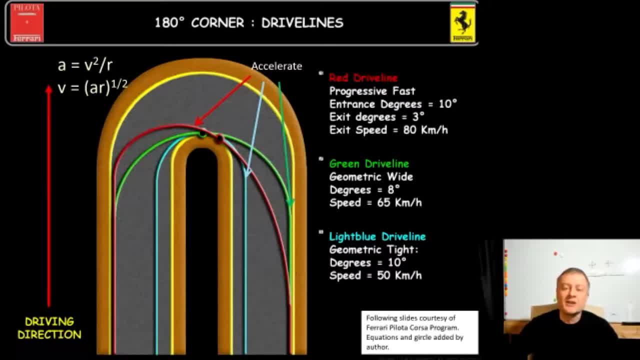 the track and that usage of the entire track gives you the largest possible radius, which gives you the highest possible speed through that corner. so, again, one of the challenges of racing is, uh, using the full track and having the confidence to start at the very edge and, even more challenging, to finish at the very edge of the track. 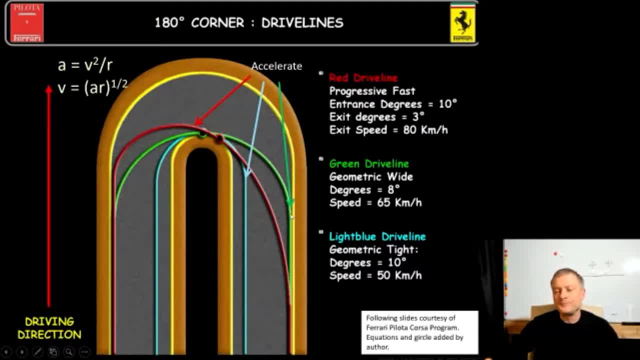 whilst trying to stay at the limit of grip. now, the optimal line through a turn um is greatly influenced by what comes after that turn. so you'll find, uh, actually, more often than not in racing we use this red line, where the initial radius is is much tighter, but the radius opens up and we get a much broader radius as we exit the turn, to allow us 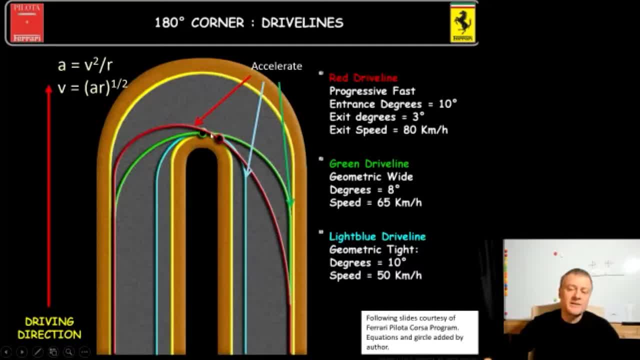 um, to spend more of a traction budget on acceleration coming out of the turn and having the highest possible exit speed, which is very important in cases where there's a long straight coming up after the turn, and so that that speed gets we, you know, pays dividends to us all the way through that straight. 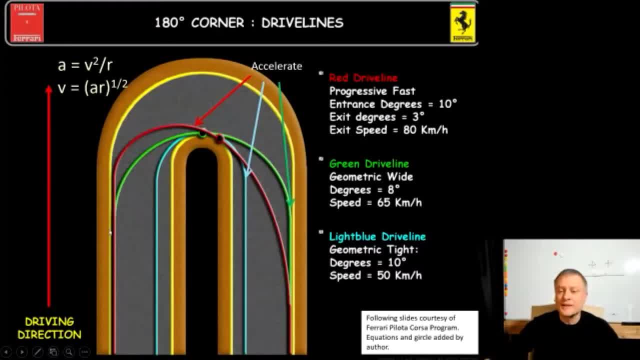 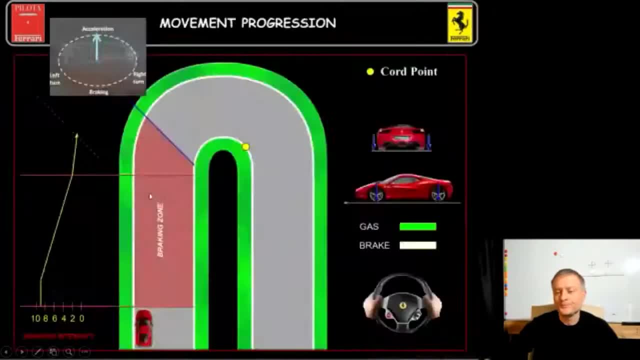 okay, so, uh, that's the briefest possible introduction to racing lines. uh, as you'll see again, usage of the entire track and trying to stay through the limit of grip on the whole, on the whole curve, is really critical. so let's look briefly what happens as you approach a corner. um and again, unlike going to get, 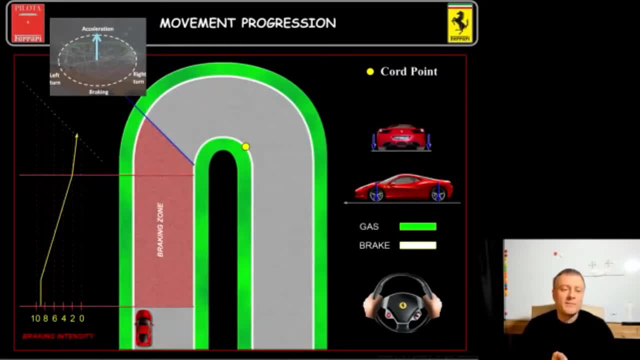 groceries. as you're, uh, approaching a corner, um in a race, of course, or racing, your foot is fully on the accelerator. you're going as fast as you can. your acceleration vector- probably engine limit- at that point is pointing straight up, or your friction vector rather, and you switch very rapidly as you. 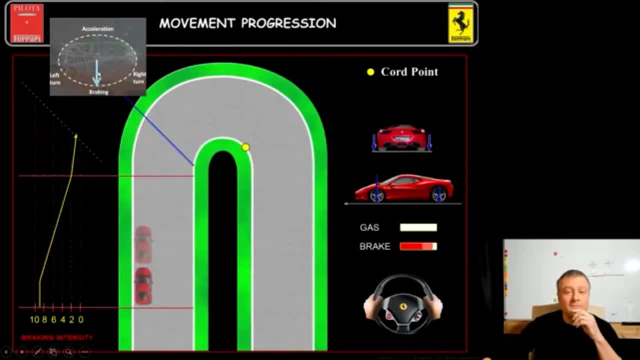 approach the braking zone from that point to braking. okay, um, again, for shortest possible lap time. you want to leave that moment until the very, very last possible moment. and uh, at that point the steering wheel is straight, your foot is hard on the brake, you're at the traction limit of braking. 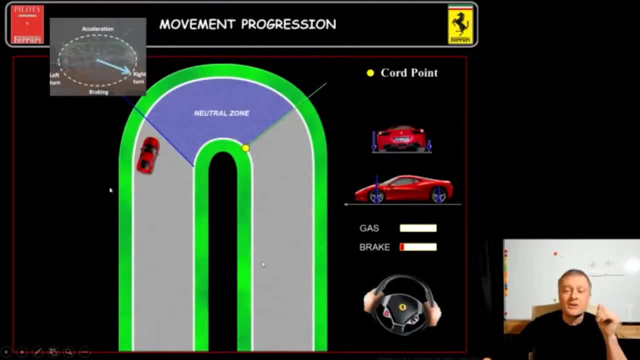 and gradually you get off the brake as you start to turn the steering wheel, as you can see what's happening with the friction vectors. you're repointing the friction vector from under braking and, ideally, keeping it on the edge of this envelope, turning it towards where it's going to be. 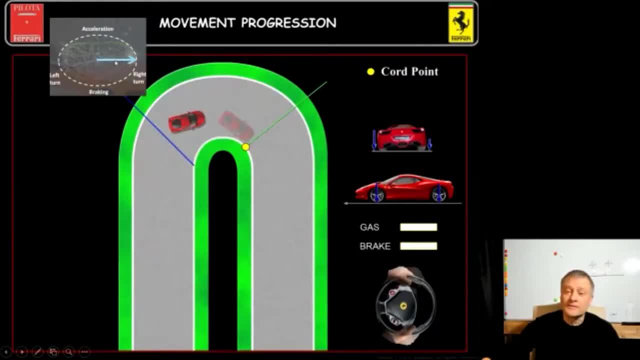 fully transverse. so now this is a frictional force to create the centripetal acceleration that you need to make the turn and, as you preach, approach the apex, which in italy they translate to cord. you get on the gas gradually right. so here, middle of the turn, steering wheel is fully turned, no bra, no brake. 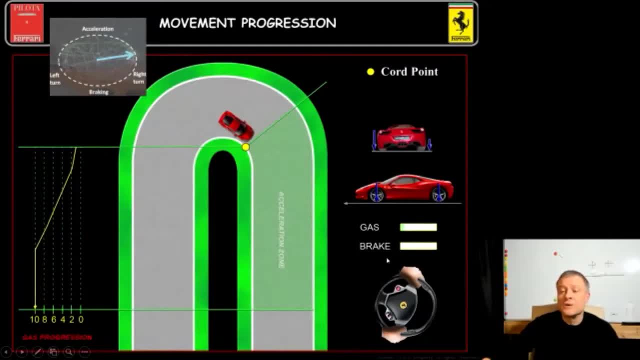 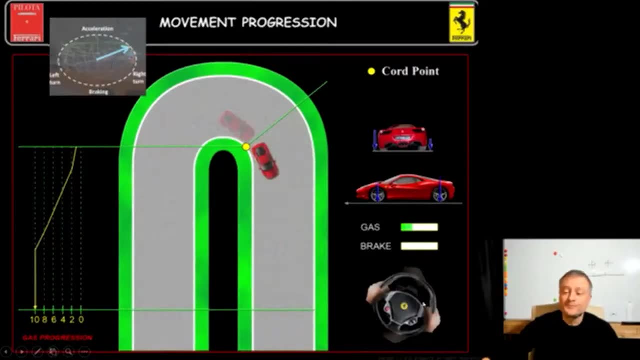 no gas. and then you gradually start to unwind the steering wheel as you start to apply gas so that again you're trading off cornering grip for acceleration grip, keep unwinding the wheel and get further and further down the gas until you're finally on the straight again in a full gas. so 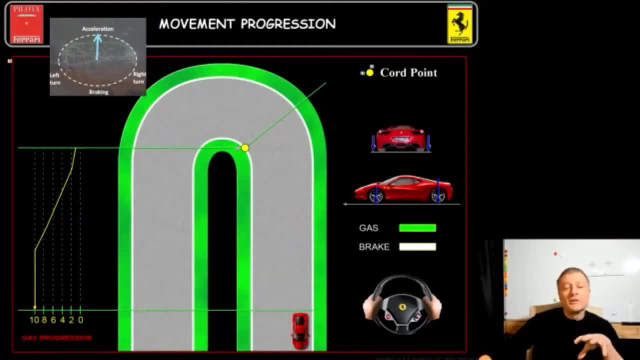 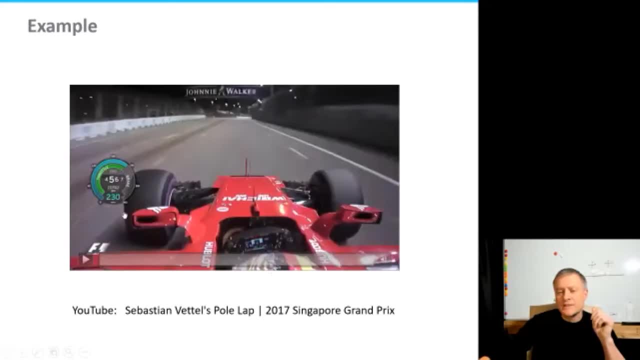 i'm going to show you um, now they understand that progression. if you look at a um a video. this is a vettel and in the formula one, ferrari, uh, in singapore 2017. um, this is an interesting video because it shows the graphic of throttle and brake. so there's this. 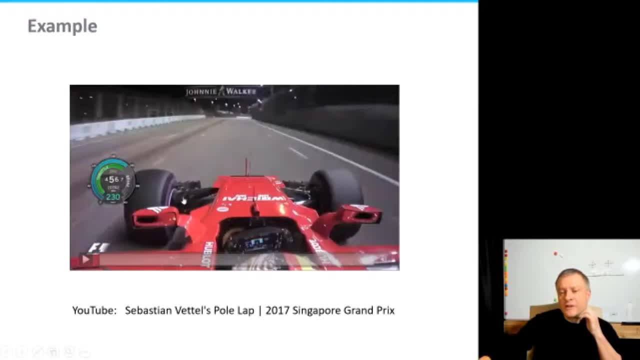 green line. that's the amount of throttle that he's putting in. i'm going to start the video on a straight, so he's a full throttle and then there's a red line that's going to be generated when he hits the brakes. so just watch a few seconds of this video, paying attention to 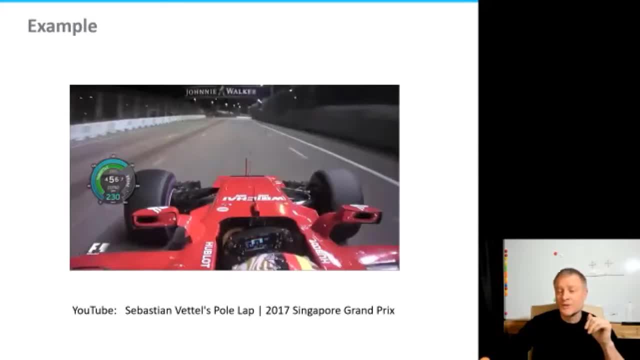 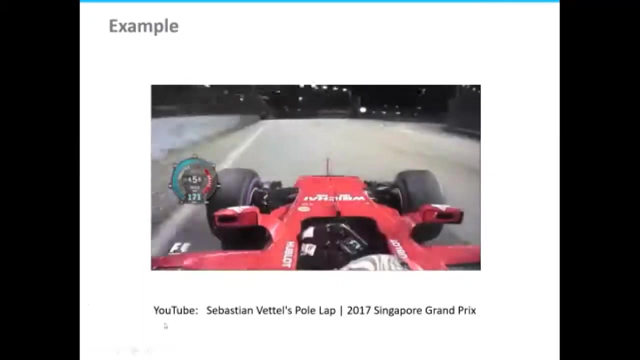 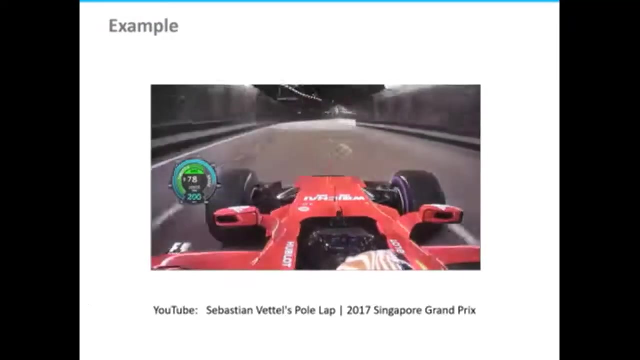 the extent to which he uses the track limits which are surrounded by concrete walls here, and the two ずi car borrowers, then all the tires can use a maintained brake on to instal. you'll see here- and his aren't just see here- as they shift over the mute um section, there is the braking. 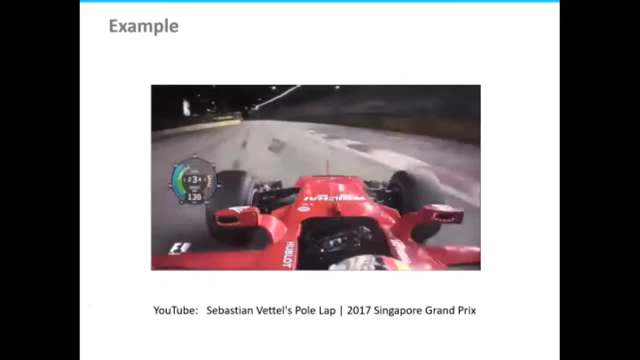 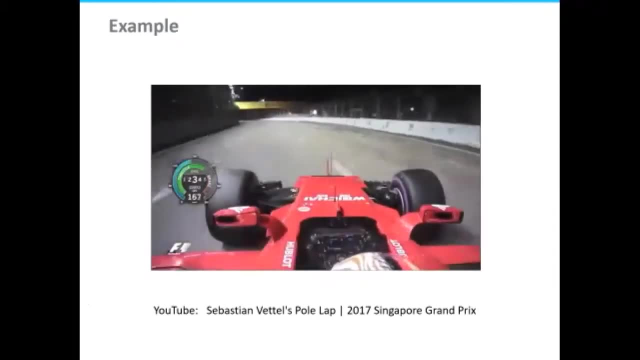 compared to get on much more than that. certainly, duel with the steering wheel, so you can see the walls, to be able to maximize the, uh, the radius of those turns. okay, apex, getting very close on the exit and again starting near the wall. apex getting back close to the wall and so forth. 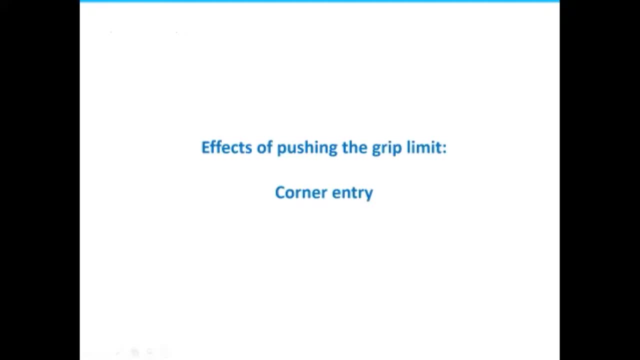 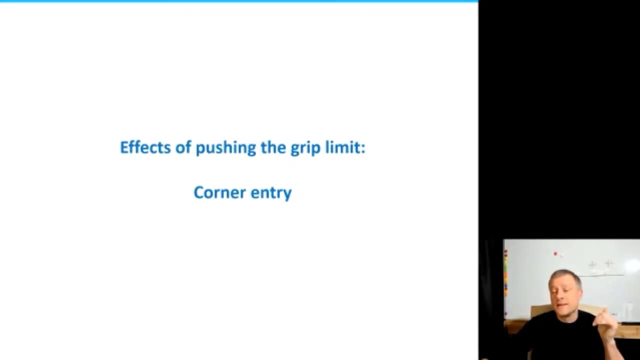 okay, so hopefully you uh get the picture there, um and again, just impressive levels of control to be able to, to get to those points and um and not hit the wall, obviously while still trying to keep the grip of the absolute limit. and this is the, the challenge that's hard to notice on television. 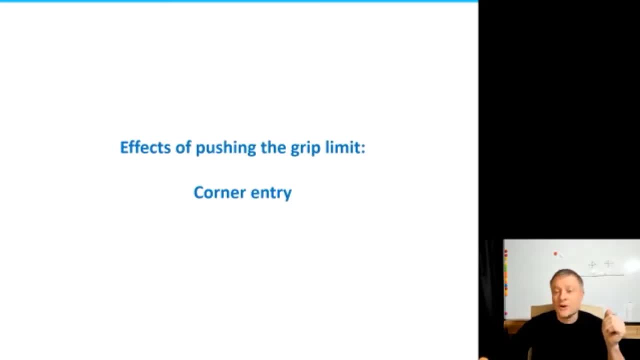 that that these racing drivers do. you know phenomenally well now what happens when we sort of get beyond the edges of that right, and as a beginner driver, uh, of course you experience all sorts of problems trying to get to that point. it doesn't look nearly as smooth as, uh, as these professional drivers make it look, and uh, so let's. 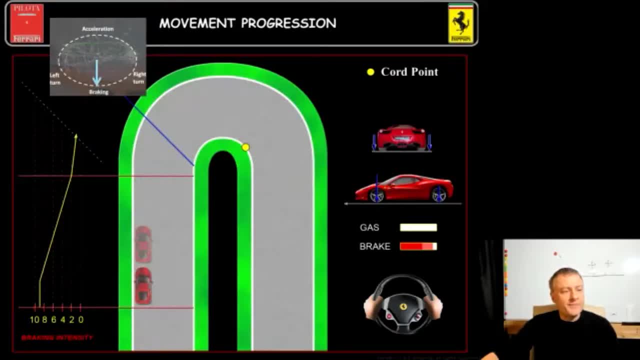 analyze what it looks like. um, you know, starting with the braking point. so in some of these tracks, we're approaching the point at which you need to hit the brakes at speeds upwards of 300 kilometers an hour, and that that's close to 100 meters per second. 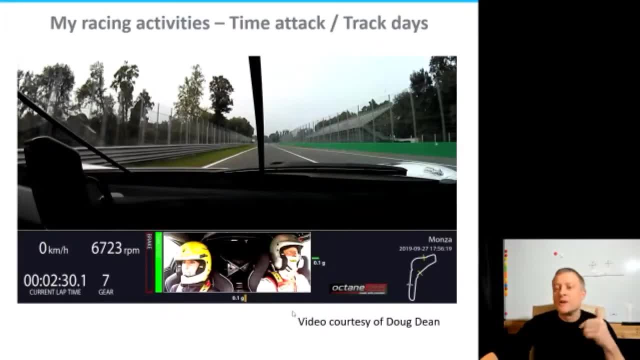 the track itself. uh, in some cases- and this is the straight at monza again, uh, followed by the first hairpin, the- the width of the track of that hairpin is maybe six meters wide right. so when you're traveling at 100 meters per second, you're trying to optimize your braking. 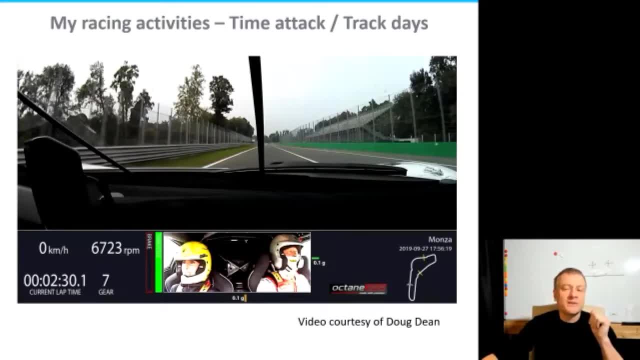 the entirety of the width of the track will go past you in about 100 milliseconds, so the the timing of the braking is incredibly critical. i'm just going to show another few seconds of video. what you can see in um this little white board in the middle is the 200 meter marker. 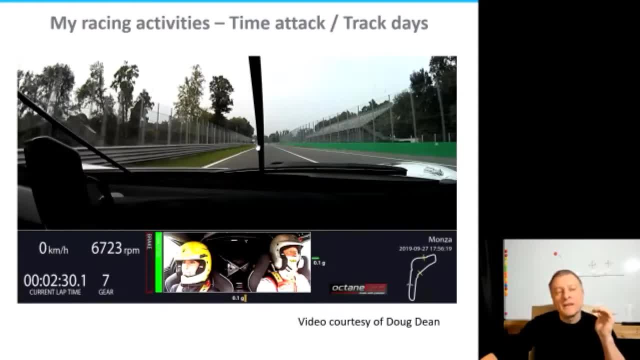 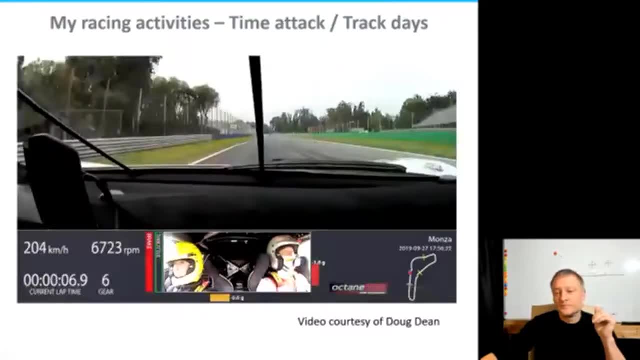 and they're spaced every 50 meters and just watch how quickly they go by, from 200 to 150 to 100.. how quickly they actually go by and how fast they're getting to the brake out and how fast they're going through the track. so we'll go through the braking points. 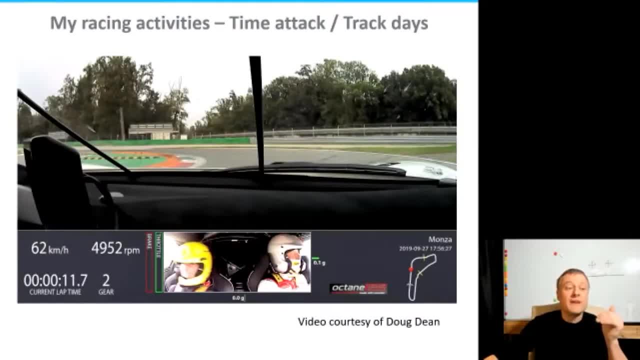 with the brakes at the right moment. uh, if there's not enough braking points, those are the proper braking points. and then, if it's a little bit faster, you get to a take-off. so you're traveling past those braking points so fast you have to see them coming up and again, hit the brakes at the right moment, uh, at monza, if you get that wrong, it'll be embarrassing because you'll end up having to go straight instead of through the chicane. if you get that wrong and knox, of course you end up in a tire waller, in the ditch or something like that again. that's one of the big challenges. is that split second timing that every- uh, every race car driver can have. 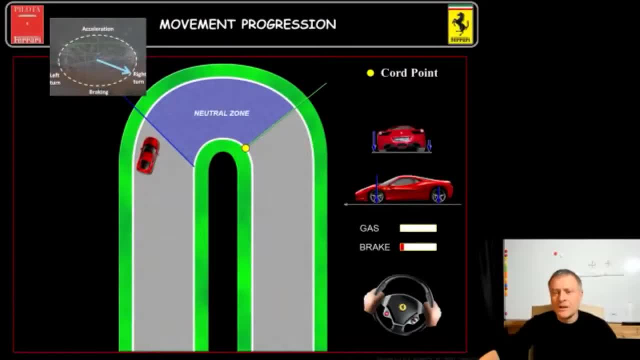 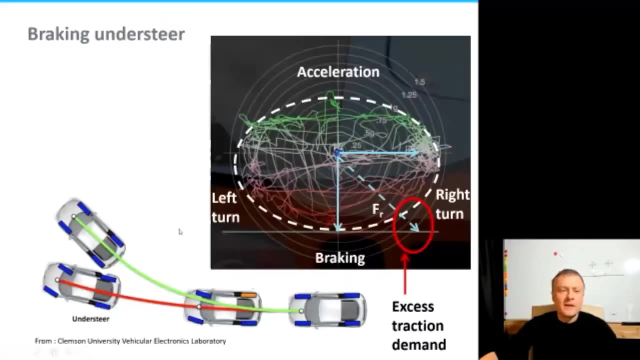 driver really needs to develop. And then, of course, there's this: this field is balanced in the turn, trying to trade off braking versus cornering and then eventually power versus cornering. So what happens if you get that wrong right? So if you, for example, leave your braking, 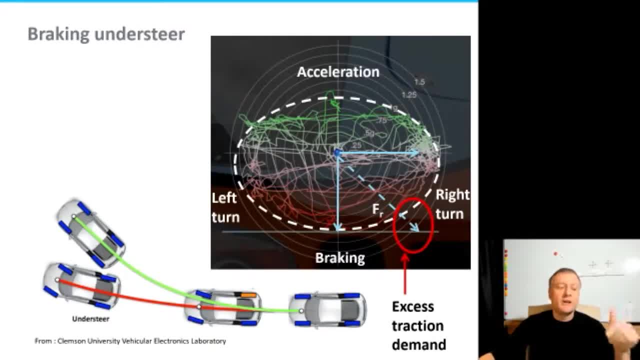 point too late and you're still relatively hard on the brakes as you approach the turn. you're going to get into a situation where you're expending all your friction right, braking right, So your coefficient of friction is being utilized to provide fully the maximum braking. 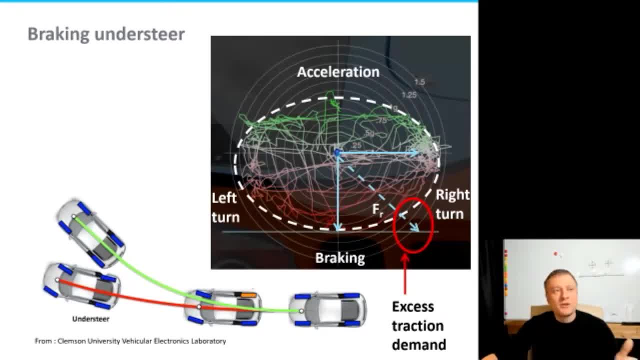 force. If, at that point, you turn the steering wheel, there will be no, no additional frictional force available to you to provide any sort of turning, Because if there was, of course you can end up with a resultant that goes outside of the maximum you know friction coefficient. 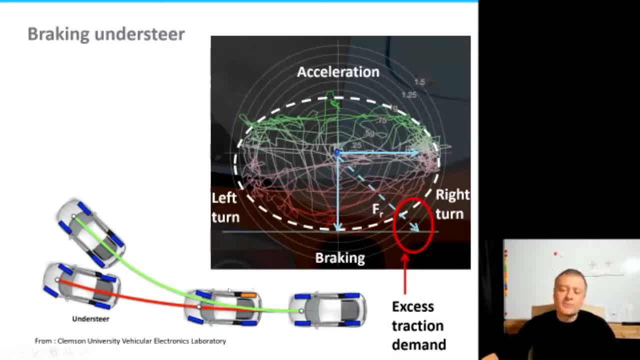 and that's, that's just not going to happen Now under braking, both because the front axle is taking the majority of the braking force and because turning in the car provides the highest load on the front axle. What happens under braking if you're, if you're trying to exceed the traction budget, is you get? 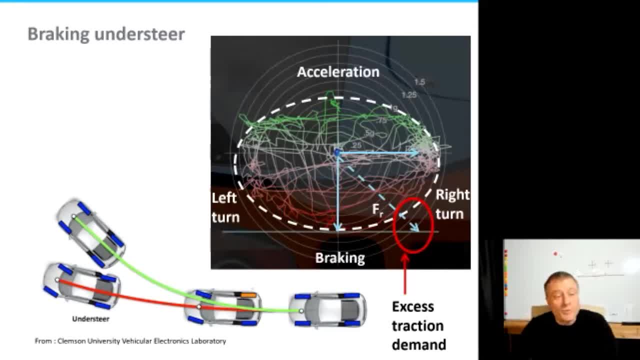 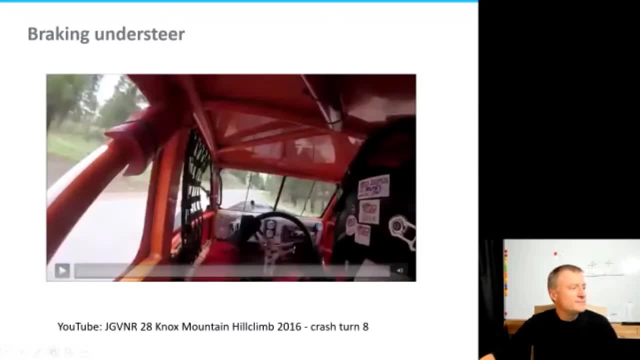 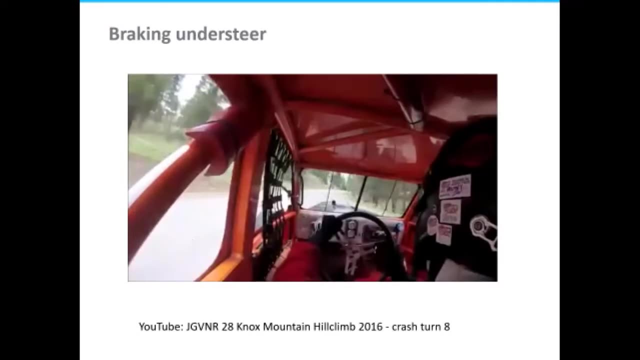 what's called understeer. Now, understeer is where the slip angle of the front wheels exceeds the rear wheels, and oversteer is the opposite. And here's what understeer looks like. Okay, this is one of my, my fellow competitors at Knox, coming into Turn A just a little bit too fast. 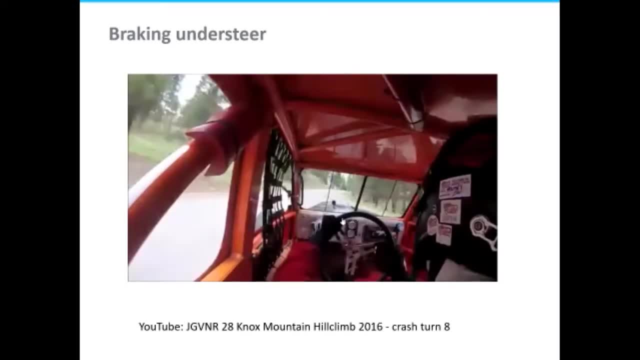 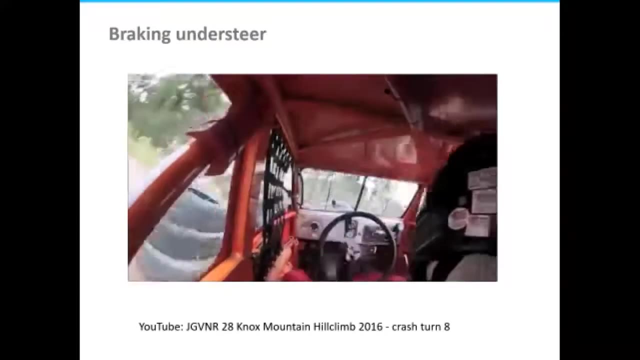 And just watch in the video, you'll see from the inside and outside. watch the steering wheel right, Because you can see what he's trying to do And because he's on the brakes a little too late, it's just not going to work. So he tries to turn in no luck into the tire wall. And if you 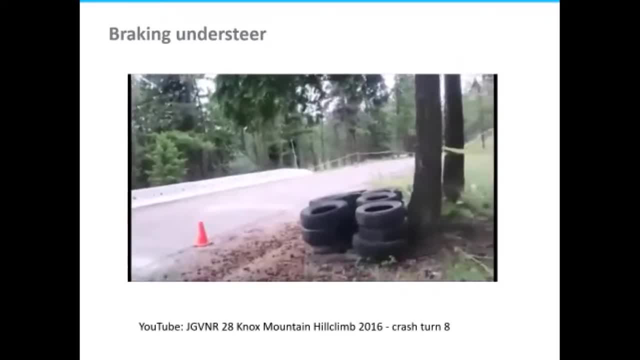 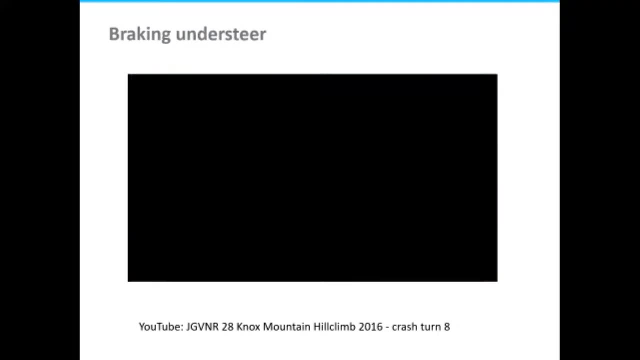 see it from outside. you'll see it. you'll see his front wheels. you'll see his front wheels again turning into the turn. But that turning of the front wheels does absolutely nothing And the car basically continues straight. So that's braking understeer And it's one of the 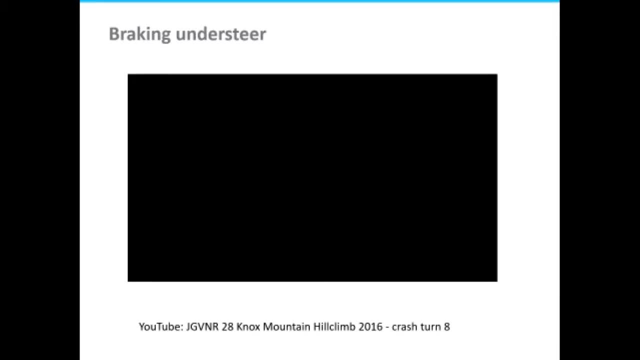 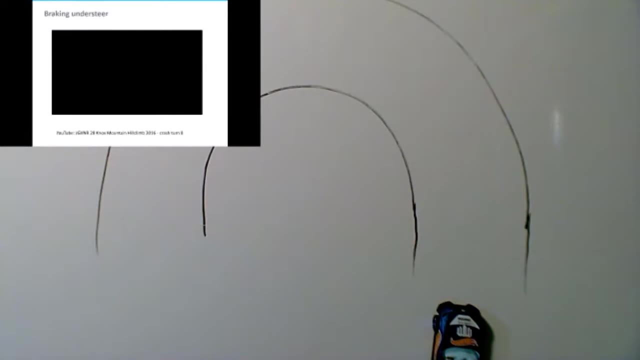 things that can happen in a car, assuming that you're braking hard way too late into a turn. Now the problem is actually compounded, And it's compounded because of this issue. Okay, So let me grab the pen here. Hopefully you can see my little Hot Wheels car trying to go around a. 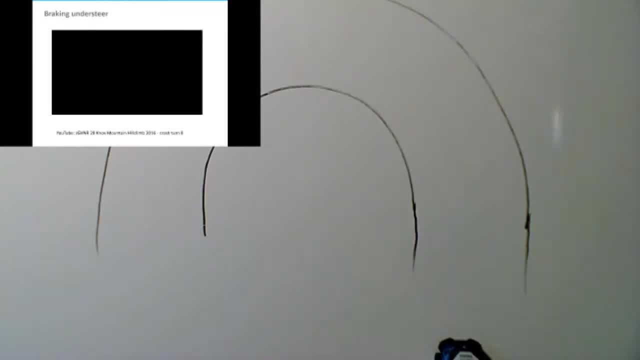 track. Now it's starting in this direction, into the track right, And it's going to go around and come out this side. Okay, So it's going through a corner And, yes, of course there's some centripetal force towards the center of the turn that has to act to keep the car from sliding. 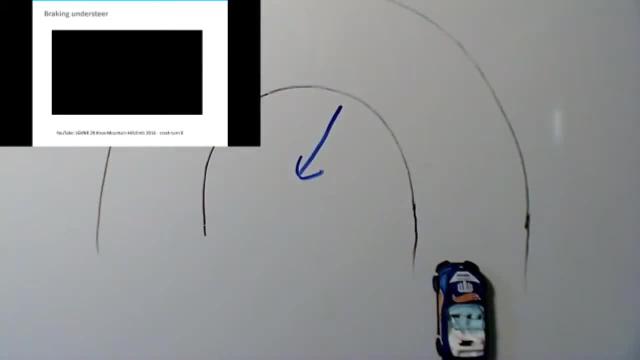 off the road. But if you look at this in the frame of the car, you'll see that the car is in this direction. So the car is also being rotated around its polar axis right. Some forces have to be used to effectively take the car and rotate it from that position to this position. 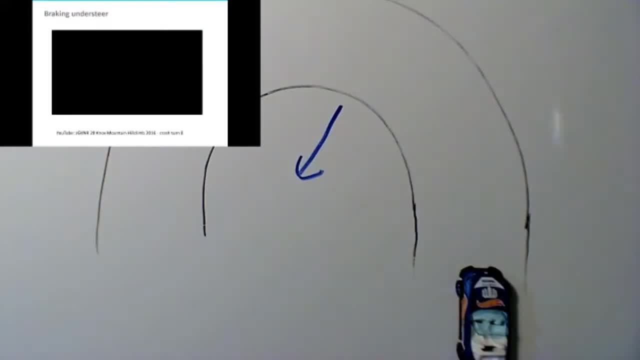 And what happens? to do that, of course there's a moment that is required. That moment is related to the, the, the, the polar moment of inertia of the car, And a force couple needs to be created to rotate the car around that point, And that's at the beginning of the turn. 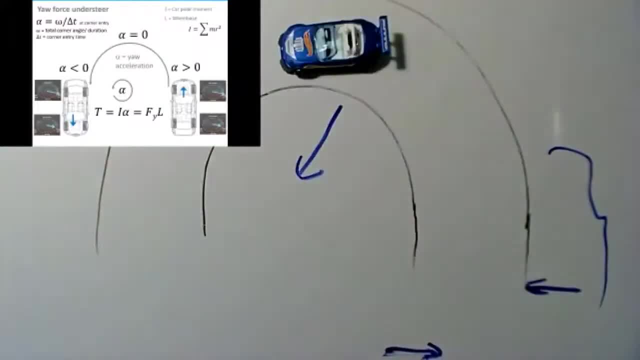 The forces are going to look that way. There's zero here, right? Because what's happening is there's some angular acceleration that's greater than zero at the beginning, There's zero angular acceleration Whoops In the middle of the turn And there's some negative angular deceleration of the exit of the turn. 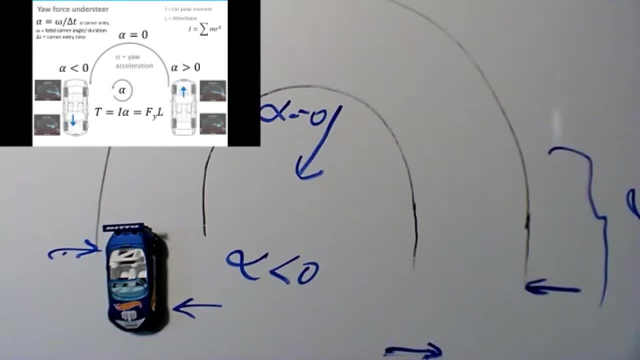 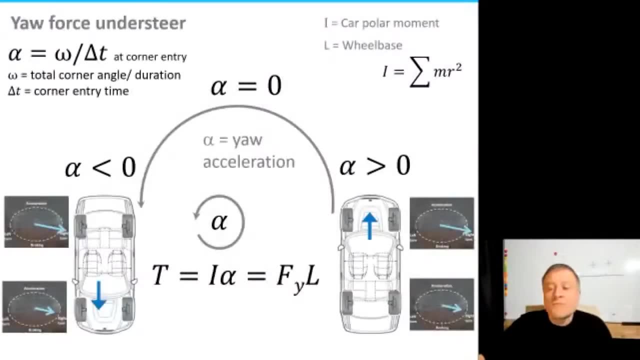 right. Where now to undo that rotation, there's a force couple pointing in this direction. Okay, so what you end up with is an additional torque requirement that's generated by this force couple applied to the front and rear axle, And again, that's related to. 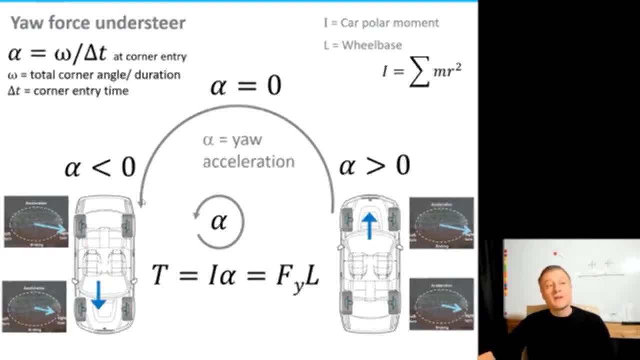 how much angular velocity is required of the car. So, in terms of rotating again around its polar axis, that angular velocity is going to be a function of the number of degrees of the turn and how long the car spends in the turn And the angular acceleration required at the beginning and then deceleration at 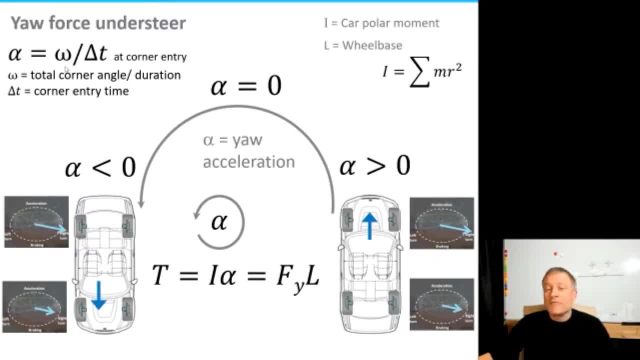 the end is going to be related to that velocity you know, divided by how much time the driver spends getting the car rotated into that, you know, into that angular velocity. So at the entrance of the turn there's now this additional requirement of the front axle. 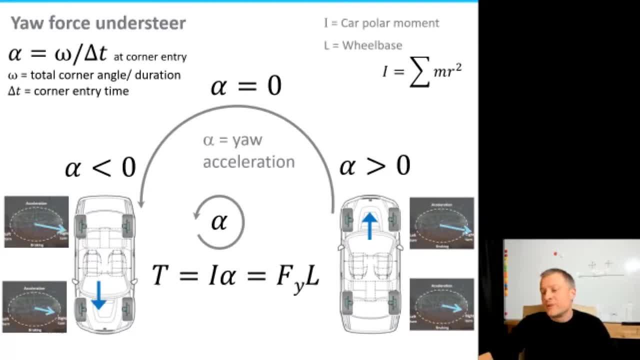 that will tend to quickly push the required friction force of the front axle outside the the traction envelope And of course makes life a little easier for the rear axle right, Because that force and then is in the direction opposite to the centripetal force. 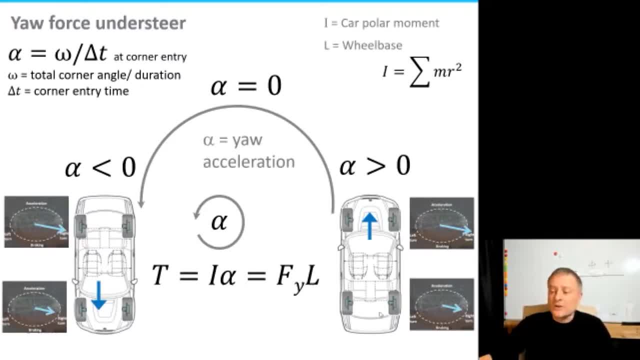 required to put the car around the turn. So this effect tends to create corner entry understeer and corner exit oversteer, And almost all race cars will suffer from those two effects, partly for this reason and partly because of the way that braking and power are applied. 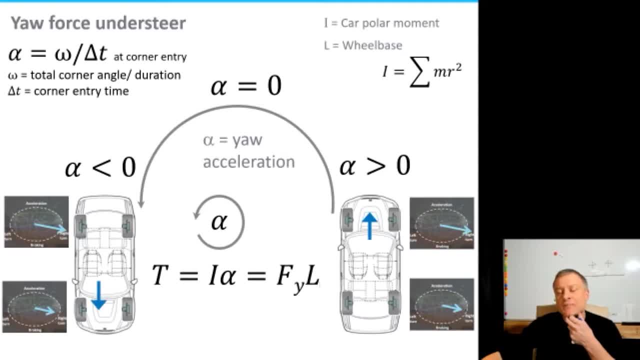 Some things to consider here, and you'll hear racing drivers talk about, you know, settling the car into the turn or getting the car rotated. A good driver will maximize this delta T right. So if you're going into a turn and you just 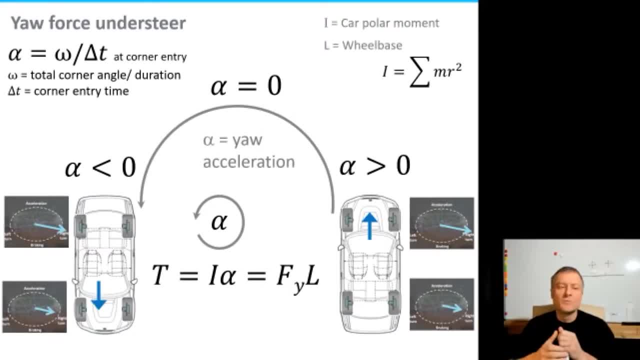 suddenly turn the steering wheel as far as you can. that will almost certainly create understeer. okay, So understeer and corner entry for beginner drivers can be a function not necessarily of the car setup but of how they drive if they're a little bit too abrupt with the wheel. And a good 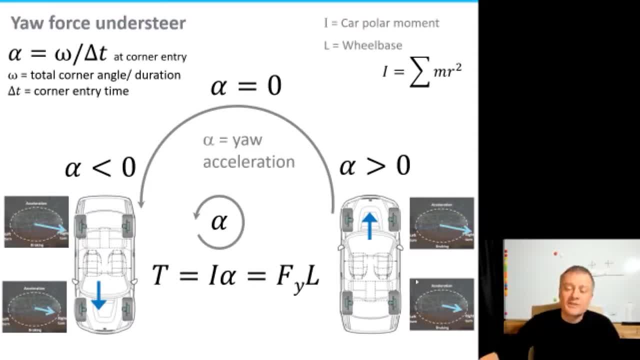 driver will try to get the car turned in gradually to avoid suffering this effect. Now, this effect, of course, is much more pronounced on sharp corners as opposed to what you tend to see in very large tracks. But in some of the racing that I do, you can definitely get you know. 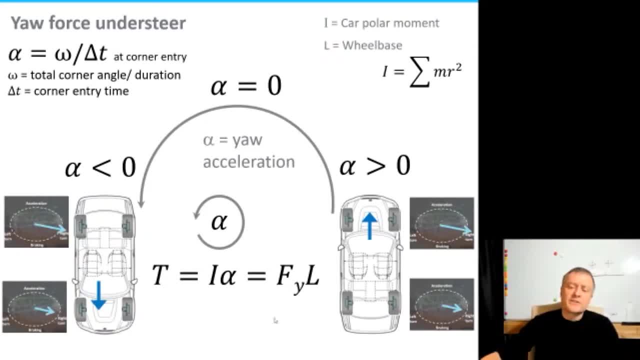 sense this happening. The other thing to consider, of course, is this effect is related to the moment of inertia of the car, And the polar moment of the car is something that every car designer tries to minimize by moving as much of the car's mass. 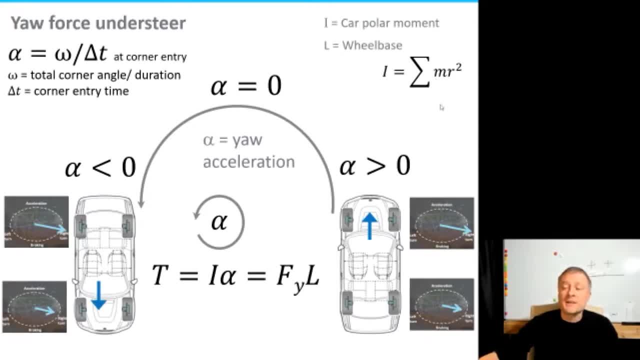 towards the center right. The polar moment of the car, of course, is the sum of all the masses times the distance squared to the center of rotation. So doing things like moving the engine back, moving the passenger and driver's seat back in the car- which you can do in a two-seater- 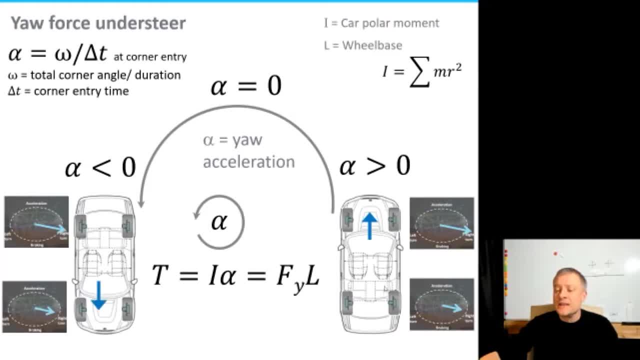 not so easy to do in a four-seater, or placing the engine in the middle of the car, which is, you know, what Ferrari and Lamborghini and other performance car manufacturers do, as well as Formula One cars. That all reduces your polar moment and actually brings with it other benefits that I won't get. 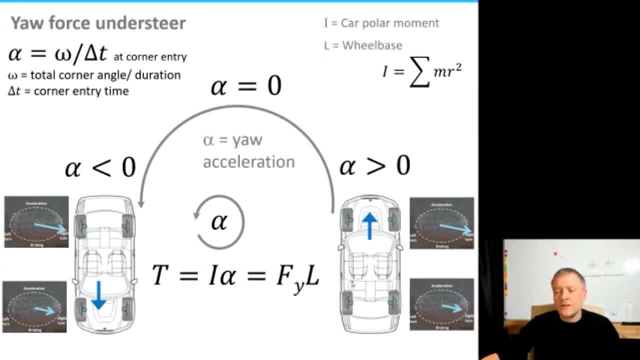 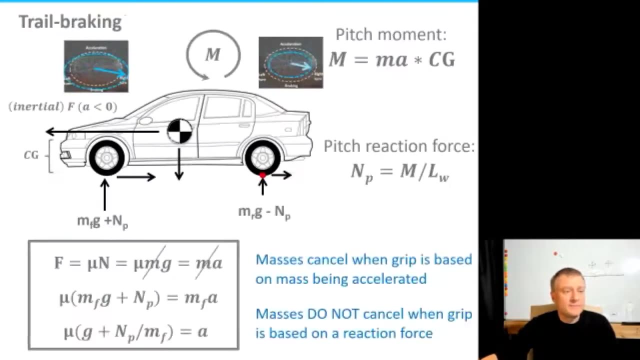 into here. So all of this, yeah, leads to corner entry, understeer, right. So, as racing drivers, how do we counteract that? Well, one technique that we have for counteracting that is called trail braking, As I've mentioned. you know, if you're hard on the brakes entering a turn, 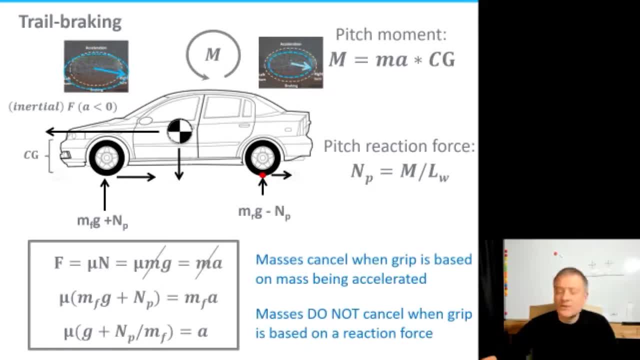 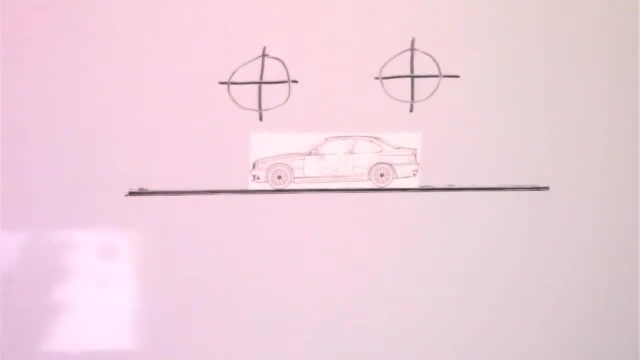 you will tend to exceed the traction budget there, But there's actually a nice- let me switch to a different graphic here. there's a nice balance where you can be a little bit on the brakes okay. So if you look at, you know. 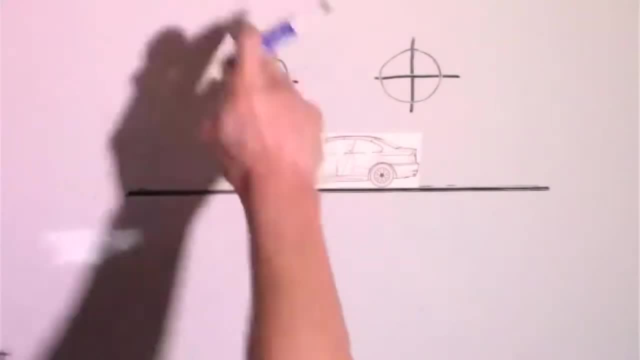 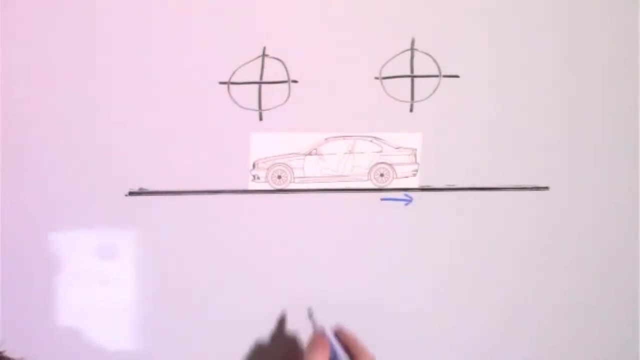 let's call these two things here: the traction circle for the front and for the rear axle. And of course let's say there's a braking force on the rear axle. there's a bigger braking force in the front axle, but now you've reduced the braking force to where. 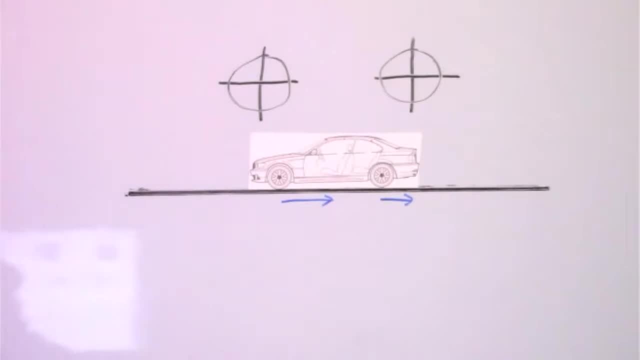 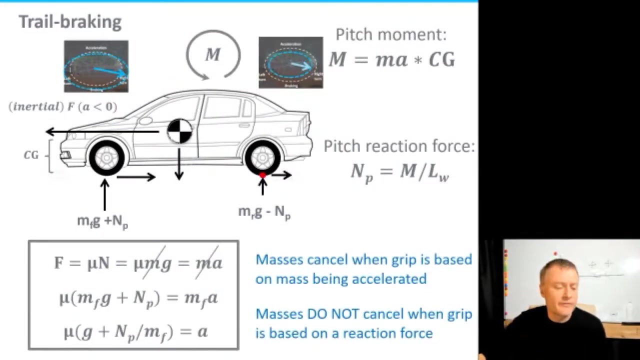 you're no longer exceeding the traction envelope, Those forces will generate a roll moment to the car right. Let me go back to the slides for a sec. So- and I've taken some liberties here- I've turned accelerations into inertial forces to make this into more of a statics problem. 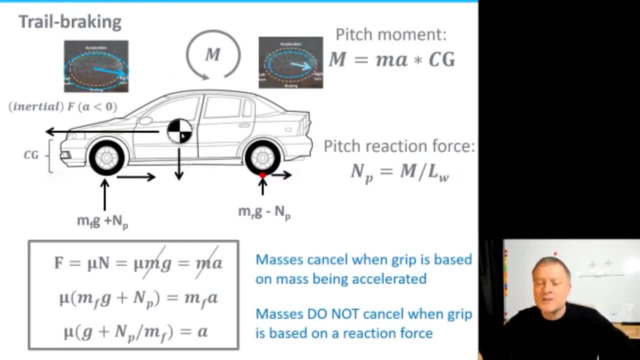 just for people's intuition, But obviously, as you try to decelerate a car, there's a, you know, a reverse acceleration, so a deceleration which in a statics problem you can think of it as a forward inertial force, And that force has to be counteracted obviously. 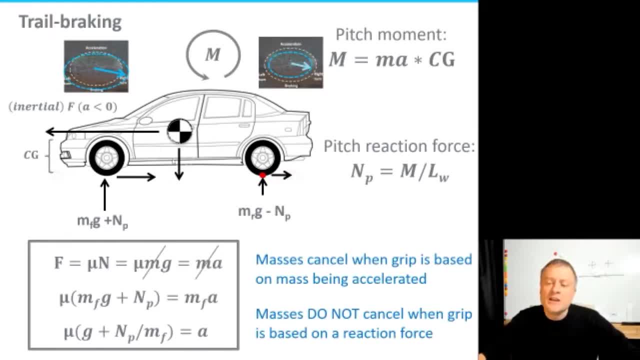 in the horizontal direction by the frictional force of the wheels, But that force, since it's applied to the center of gravity of the car, creates a pitching moment to the car and tends to pitch the car forward, And anyone that's driven a car will have experienced this, even in a road. 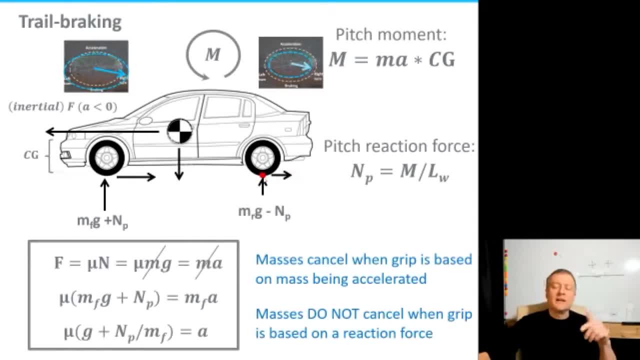 car. Now, if we take moments around the rear contact point of the, the contact point of the car right, we'll see that that pitching moment has to be counteracted by an additional normal force of the front wheels right. And in fact, if you then take moments around the front wheel, 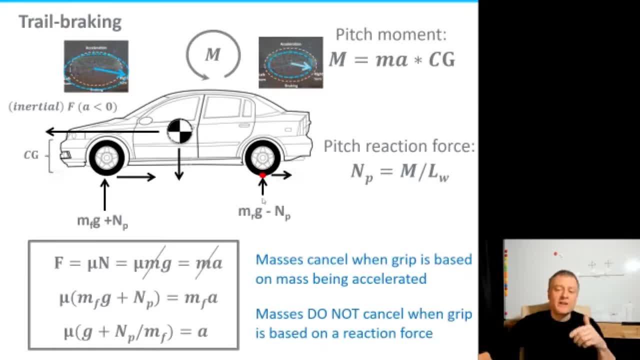 you find there's a decrease in the normal force of the rear wheels. In other words, there's additional force, additional normal force at the front that is not created by additional mass. right Now, with, with you know, using F equals mu n, right, If we say, well, let's get the. 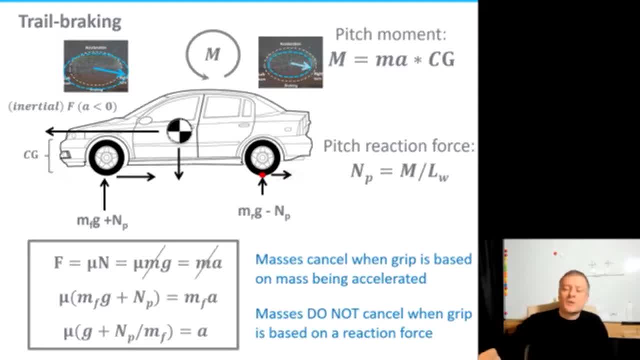 stick better. let's put more weight on the front axle. that doesn't work right, Because the mass being accelerated at the front of the car obviously would increase along with the extra weight, And- and that doesn't do you any good- it doesn't actually change the available the. 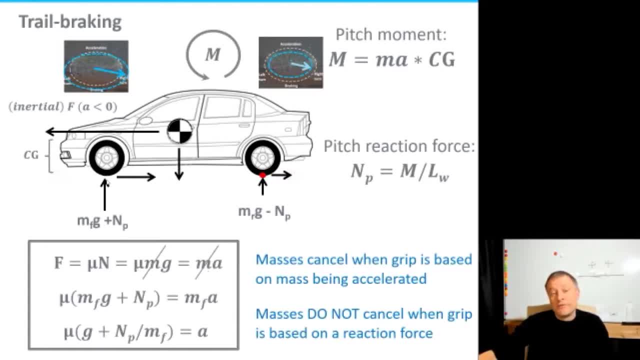 available acceleration, But increasing the normal force without changing the mass being accelerated at the front of the car- so in other words, without actually changing the mass of the car- does lead to additional acceleration. Okay, so let's go back to the board for a second. 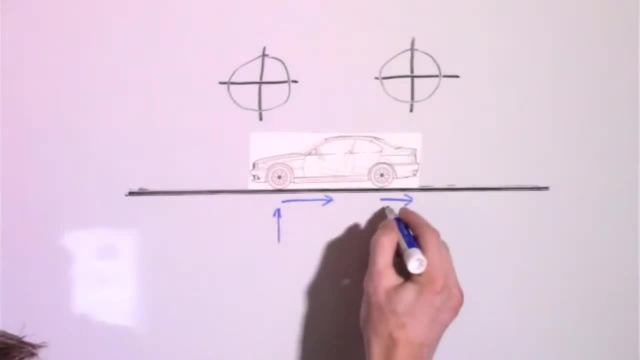 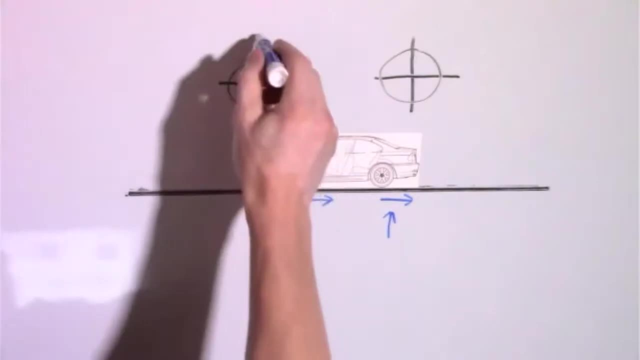 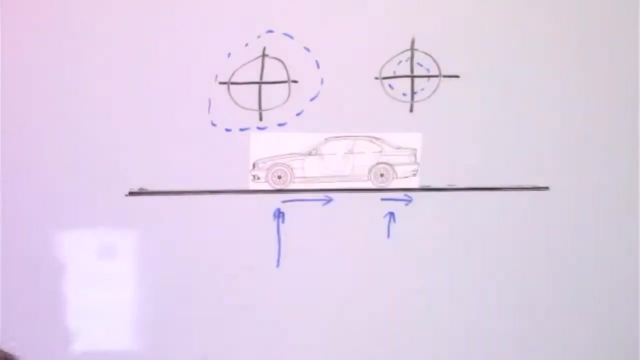 This additional normal force, right? which? so it's? basically, you get a large normal force in the front, a small normal force at the back, does two things And in fact, effectively expands the traction envelope for the front axle and contracts it for the rear axle. okay, Allowing. 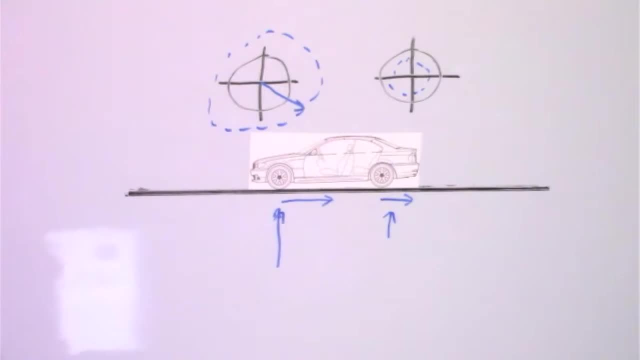 greater total frictional forces so that you can combine your braking and turning forces and get get an overall- you know, lower slip angle in the front than you would have the rear and and get the car turned in. okay, This depends on a number of factors. You can imagine that the extent to which the braking 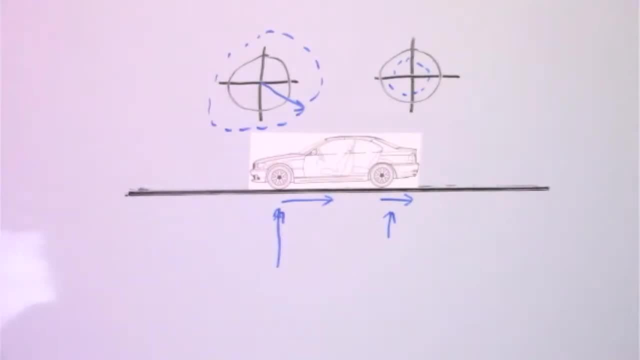 has to come from the front axle is part of that. Now, what you don't have in a road car that most, most race cars have, is something called a brake bias adjustment, where you can change how much a front axle provides a braking force versus the rear axle, And I suspect this effect 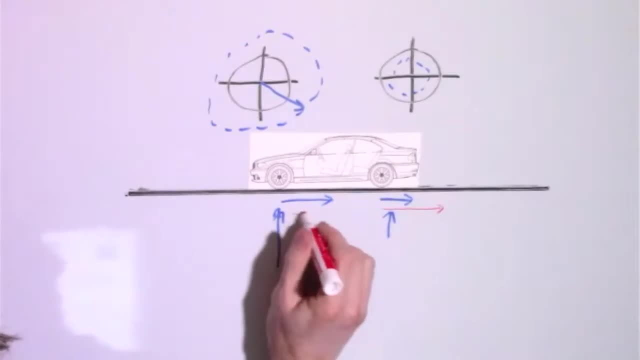 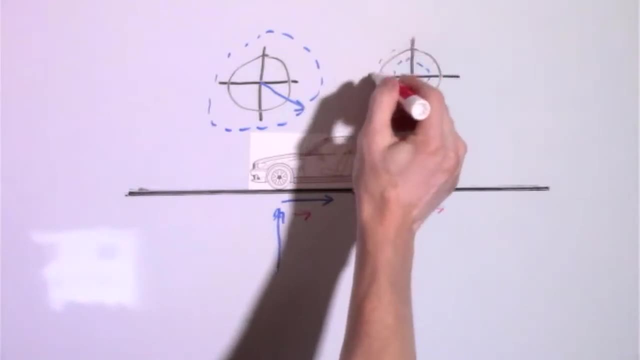 is very high because, you can see, the rear axle is now dramatically increased by, you know, increasing the frictional force of the rear axle, Although in that situation you rapidly get into a problem where you're still sorry, you're still decreasing the size of the rear axle traction. 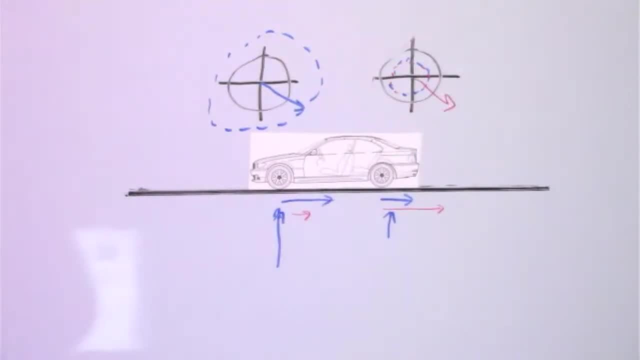 circle, but now increasing the braking force, And you'll very soon exceed the grip limits of the rear axle. And what happens then, of course, is you have something like an inverted pendulum. your front axle is stuck to the road, your rear axle is free to translate, because no additional 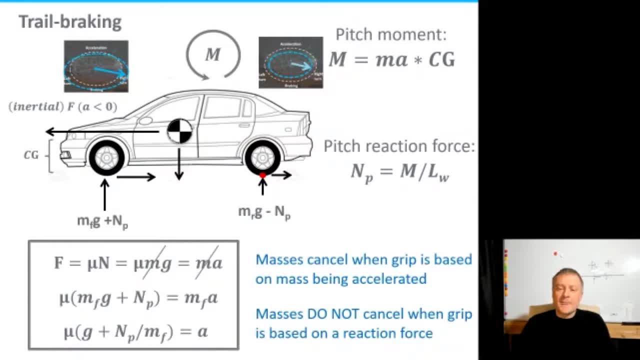 friction is required to prevent translation, and and the inertial forces are facing forward, and now you have an inverted pendulum and the car swaps ends. so of course that's why you can't adjust brake balance in your road cars, because if you accidentally put it to rearward you would 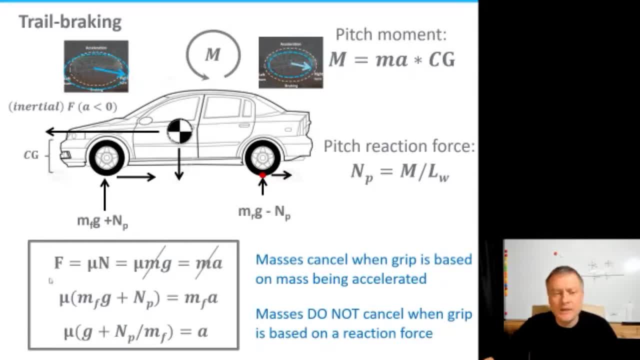 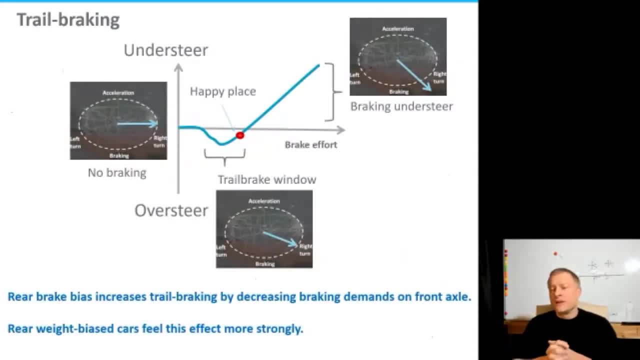 spin the car just coming up to a stop sign. okay, race drivers do have the ability to adjust that to maximize performance. so, again, one of the the cool bits that it's really really satisfying feeling this on a track is this ability to trade understeer for oversteer by how you apply throttle. 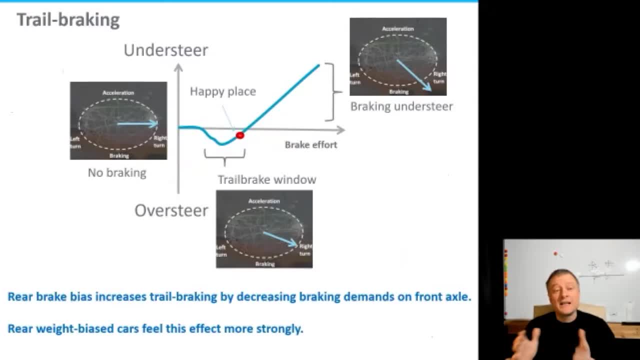 and brake, changing the the way the moments are applied between the two axles, you know, and shifting a little bit that moment and the reaction force from that moment onto the front axle to get better grip entering a turn. so in fact, at least for for my cars, there's this nice little trail brake window where you start to get a bit of. 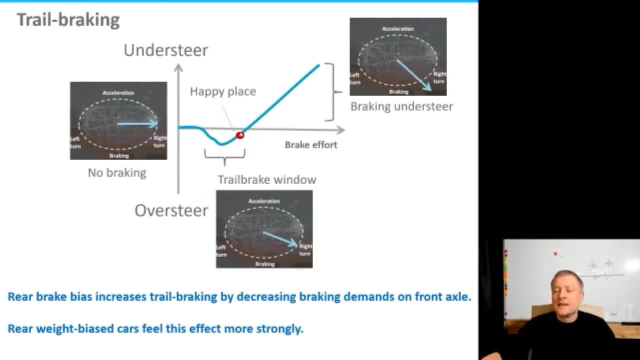 rotation of the car under a slight amount of brake, and as you brake harder and harder, of course, then you start to get into braking understeer potentially. so you're trying to find a nice balance where you've expanded the traction circle of the front axle enough that you get a good turn. 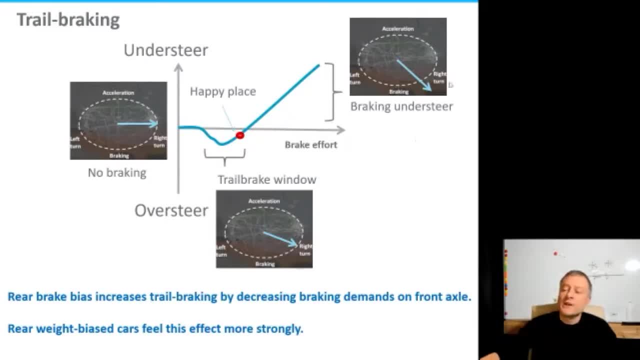 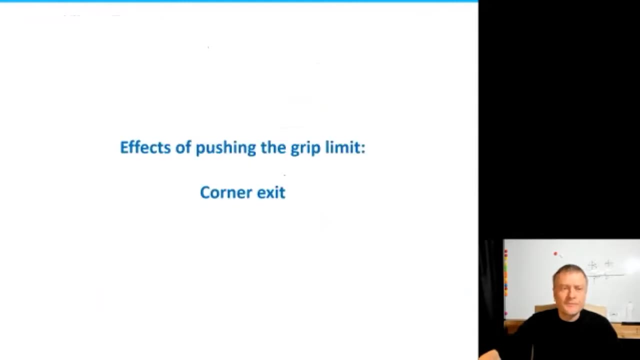 in of the car, but you don't apply so much brake that you start to exceed and get to understeer. so again, just give you a sense of the things you wouldn't necessarily see on tv, with the trade-offs that drivers are making as they're entering a corner. okay now, now exiting a turn, similar trade-off. 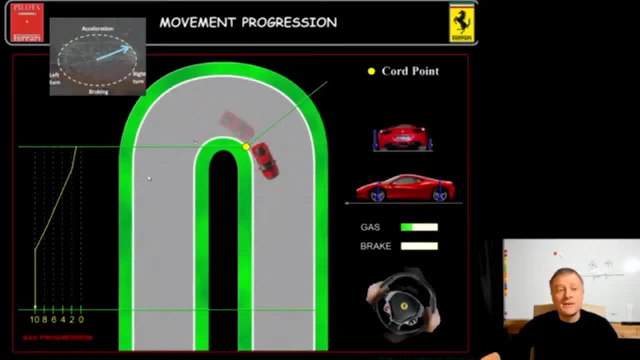 supply, right. so you're trying to now get the car accelerated again while you're still asking your tires for centripetal acceleration, right? so, in other words, they're, they're looking at, you know, for a transverse frictional force, so you're trying to slowly unwind the wheel as you apply uh gas to try to keep uh your friction. 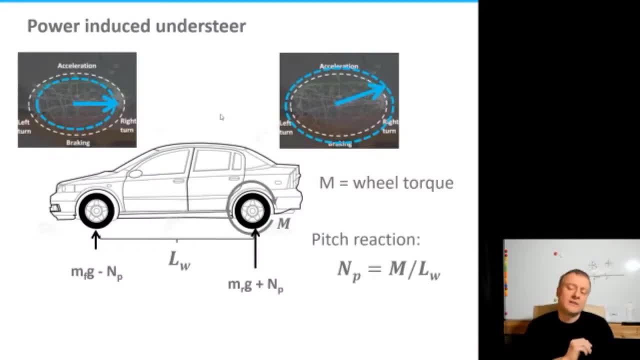 uh vector within the envelope until you're finally at full- uh, full power now again. um, two effects happen when you do that. one is there's, uh, what's called power induced understeer in corner exit. it's not a terrible thing actually, because there's so many sources of oversteer in in corner exit. 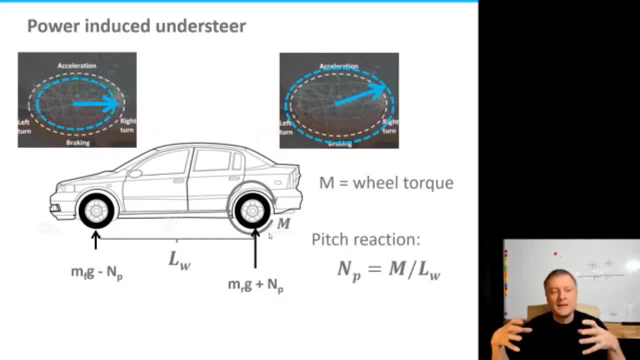 um. this effect comes from the torque that the wheels are applying right. so there's a reaction from the ground to the wheels. obviously that's what it's generating- acceleration of the car. but that course that torque is also creating a reaction of the car that is trying to make the car. 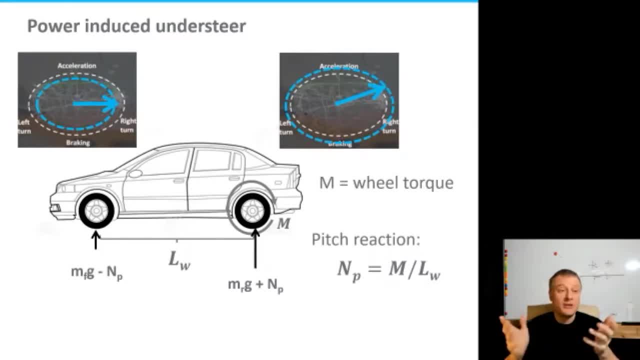 do a wheelie, not that it would obviously. well, you see, you see dragsters come close to that. so what that force is doing is decreasing- very much like trail braking, but in the opposite way: it's decreasing the load on the front wheels and increasing the load on the rear wheels. 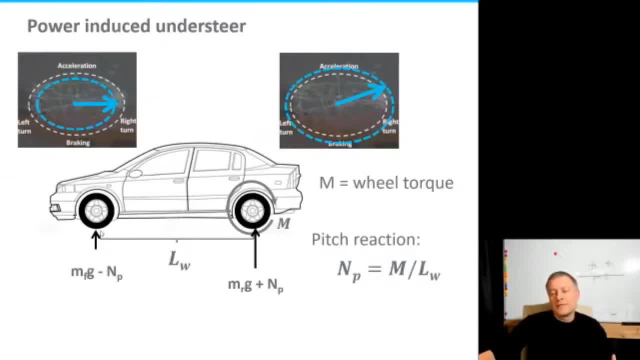 and uh helping the rear axle stick and making the front axle less likely to stick. so if you're still asking for uh cornering forces in that scenario, you will tend to understeer, okay. at the same time, there's what's known as power oversteer. now i'm 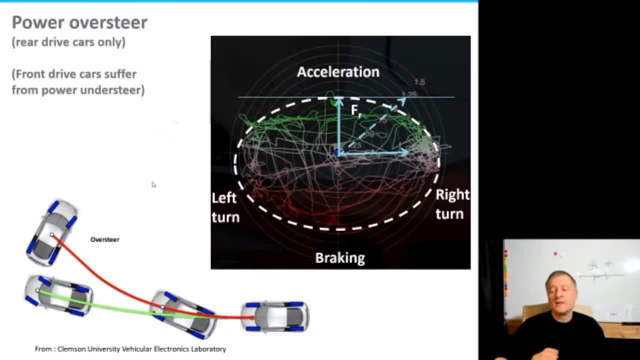 doing this all in the in the context of a rear drive car. a lot, of a lot of the race cars are- not all of them, at least mine are- and uh there that that's simply that will happen, simply as you exceed the traction budget, uh, by applying too much power to the rear wheels. 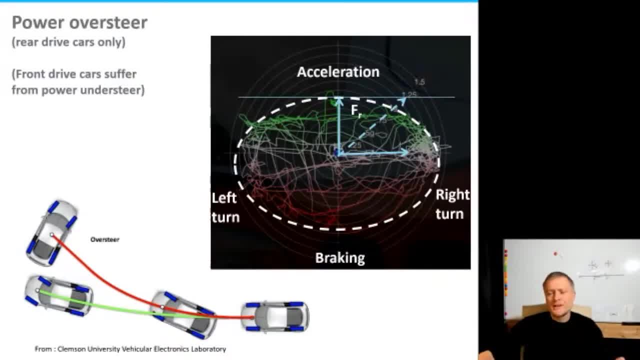 so you can't control the car. you can't control the car, it can't be controlled by the rear wheels. so that's just a very simple idea of what the power oversteer is. that's the same thing as power oversteer, and you can't control the car. uh, after the power oversteer is oversteered. 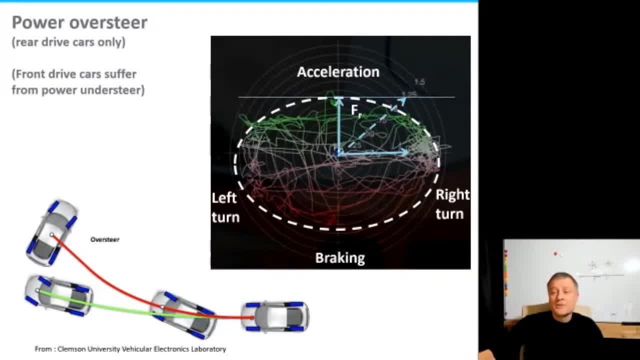 again, in most road cars it's not, you know, likely to get into this scenario because you, you know, most road car engines don't have quite enough torque to do this. but race car, race cars definitely do, and if you start to, uh, yeah, just ask too much of the rear wheels in terms of providing acceleration. 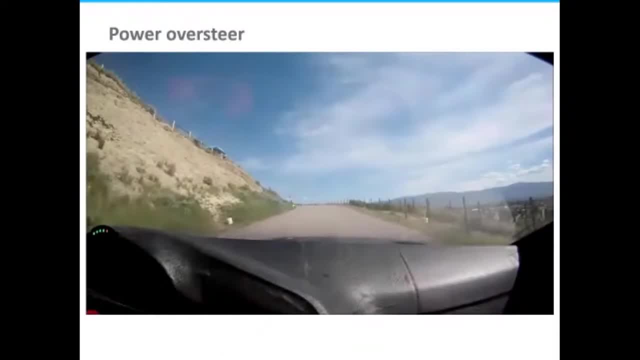 while still cornering, the car will rapidly rotate, and this is actually quite a more difficult thing to control. me at Knox. And what you're going to see is, just after this turn, as I'm a little too greedy getting on the power, the car turns as if it wants to go for a dip in the lake. before I correct it, 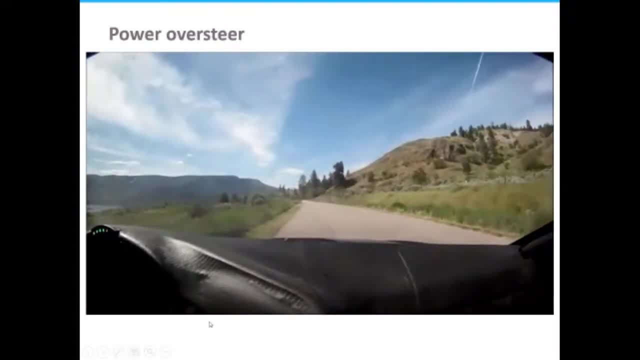 Okay, so that little wobble there I mean again easy to correct, at least in this case. But the reality is that moment probably cost me half a second in my time on that run, okay, And we're all trading tenths of a second in terms of time, so that's an expensive. 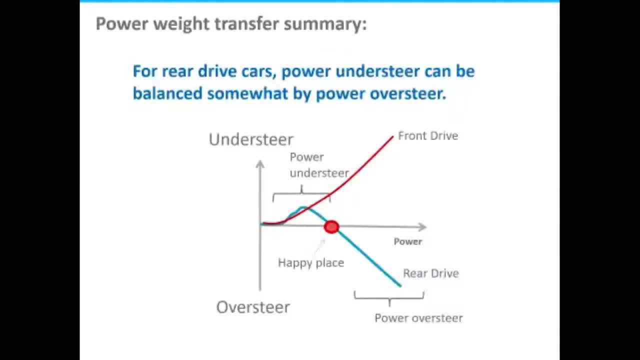 mistake to make. So for rear draft cars again, just like in corner entry, in corner exit, you're balancing multiple effects, right, You're balancing some power understeer and then you're balancing that with some power oversteer and hoping to get to a happy place where the car is going to. 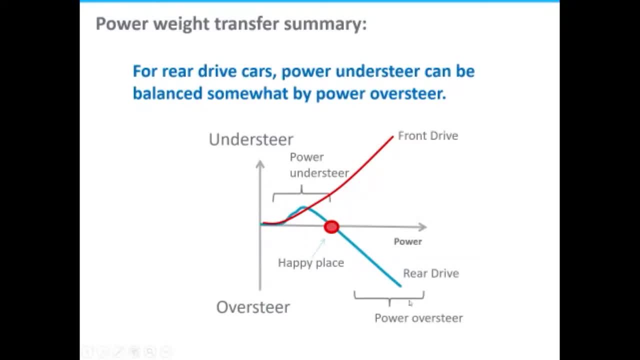 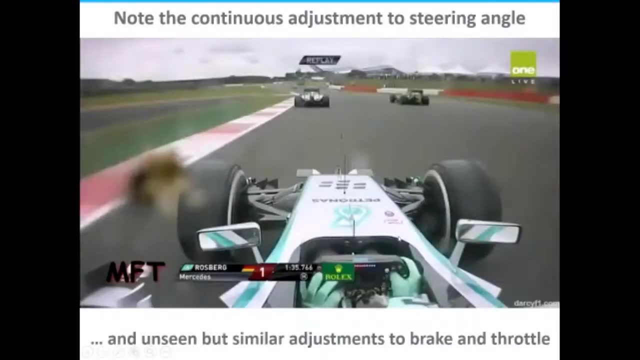 go And the car you know. the tires may be sliding somewhat right if you're at the limit of grip, but the car is staying relatively neutral. Its angle is not changing. Now I want to show you a brief video of Nico Rosberg in a Formula One car. It shows the steering wheel nicely. and what? 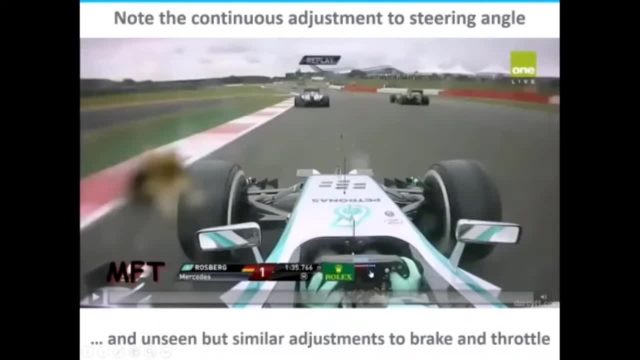 I want you to watch, for in this video are the constant adjustments that he has to make to the steering wheel when he's exiting corners, because these cars have a thousand horsepower, So the amount of torque that you can apply to the steering wheel is going to be a thousand horsepower. 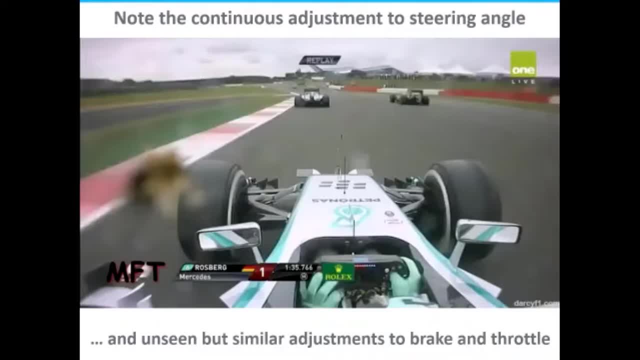 The amount of the rear wheels is enormous and I think controlling that on these cars- though I've never driven one, obviously- is incredibly finicky. So just watch this and watch him continually adjust the slip angle of the front tires to try to keep the car pointed in the right. 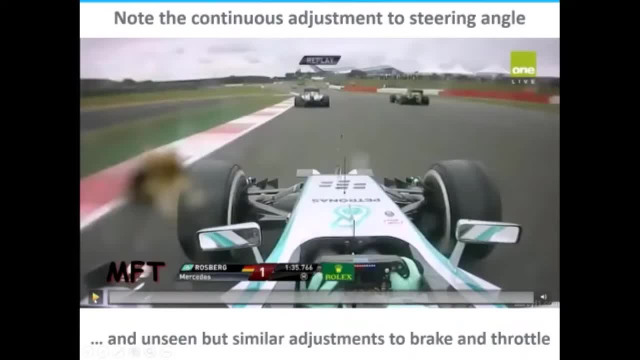 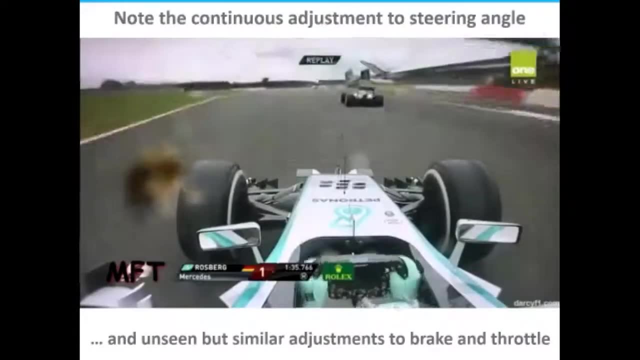 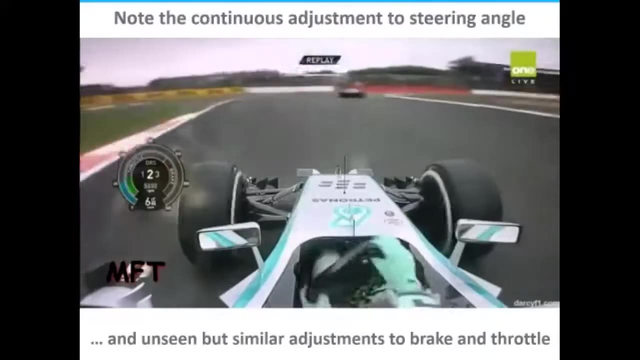 direction as the rear tires keep changing their slip angle from the power and the frictional forces induced. So a pretty smooth under corner entry. But as soon as he gets on, the power right he's. you know, look at the big changes he's. 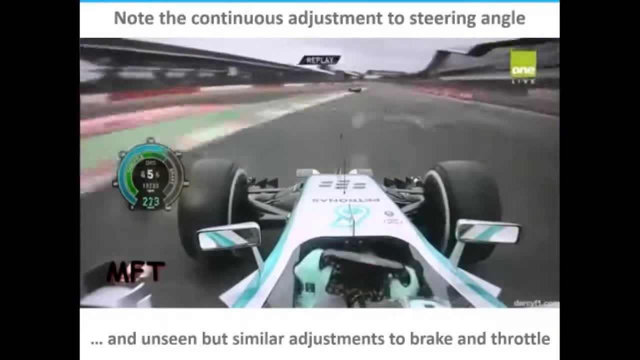 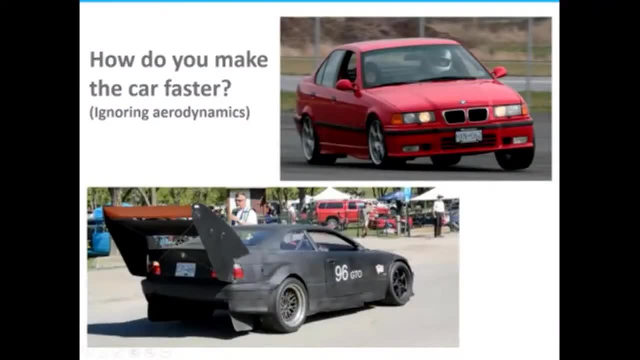 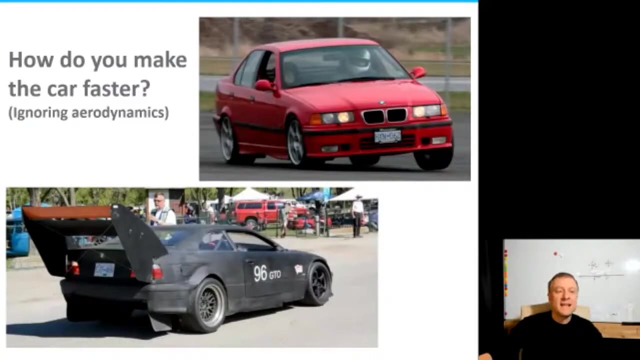 having to make to the steering wheel just to keep the car pointed in the right direction, And just that that trade-off is. I mean, what I watch is I'm impressed. I don't you know I can't make those changes that fast and that accurately. Like I said, if I get into a bit of 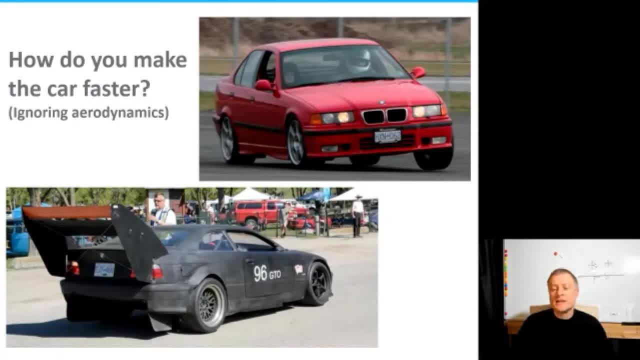 power oversteer. it usually costs me quite a bit of time and these drivers can do this on time scales that allow them to do that. So you know, I don't know if I can do that. I don't know if I can. 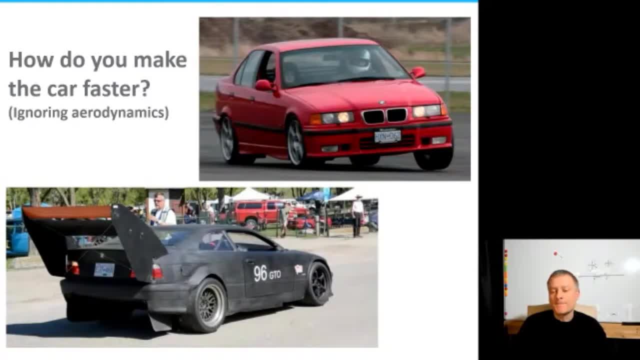 do that, But I think it's really important for them to continue to keep the car at its grip limit and maximize their lap times, or minimize their lap times, despite all those effects. So I find that incredibly impressive to watch. So that's just a little bit of a glimpse that I wanted to provide. 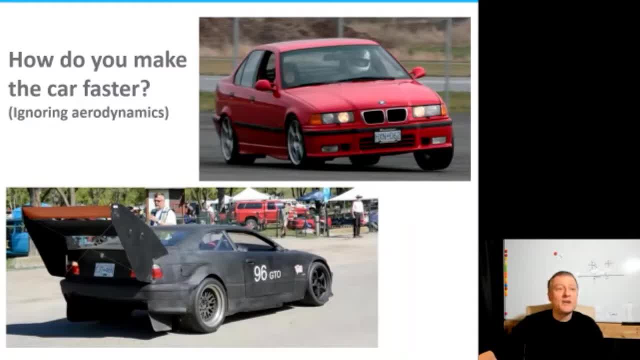 you with respect to what the drivers have to deal with and the optimizations that they need to make, And that's only you know. for the drivers in the audience, I know this is only a small fraction of the things that you do to make a car go fast around a track. 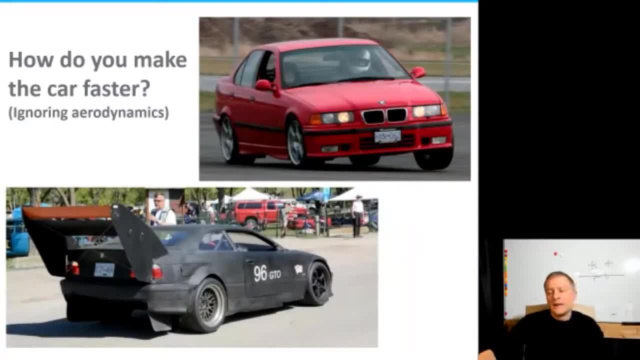 I do want to also talk a little bit about the trade-offs in car setup or car development, right, Because there's a whole other aspect to the sport which I really enjoy, which is the engineering aspect, So completely separate from the driving. how do you make a car fast And in? 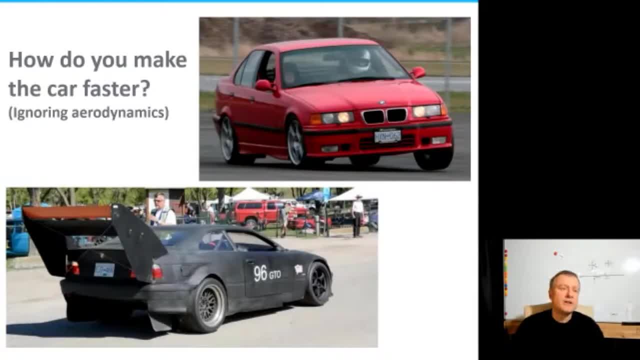 our grassroots motorsports community. how do you take a road car and convert it to a race car? right, And to understand that- and, by the way, I'm going to ignore aerodynamics, There's multiple hours of lectures that could be given on that. It's an incredibly complex topic. 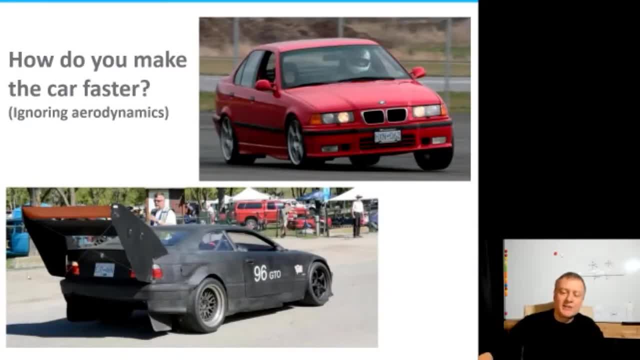 The speeds that we race at. obviously, as you can see by the giant wing I've installed on my race car, we do try to take advantage of aerodynamics, but it's the effects are not that great because the speeds are not that great In a Formula One car, 300 kilometers an hour. the aerodynamic effects. 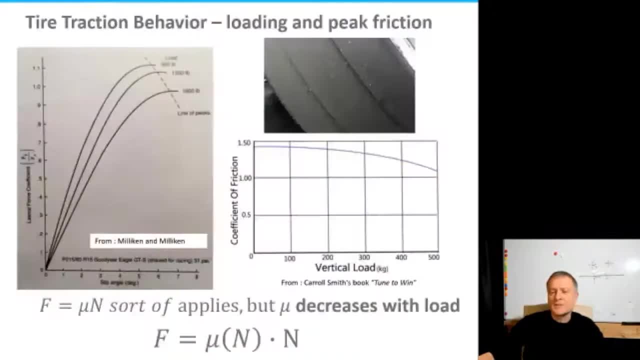 are immense, So I'm just going to ignore that for the purpose of this presentation, which means we're back to tires, right? So if the majority of the grip that you get is going to be back to tires is the mechanical grip from the tire, Now we have to start to think a little bit about what. 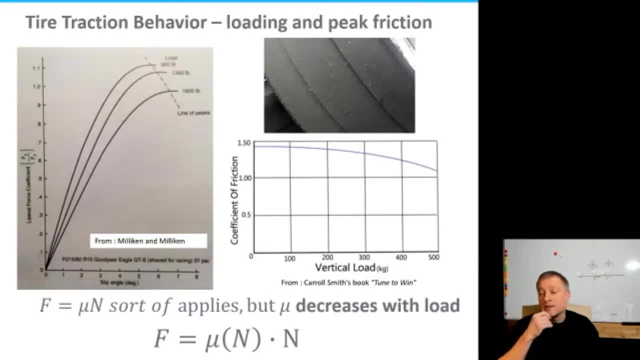 happens when you start to push that and what happens to the tire loading in the middle of a turn. So again, tires are the most complex part of a race car, in my opinion and from and the opinion of others as well, like Milliken and Milliken, as they state in the book. 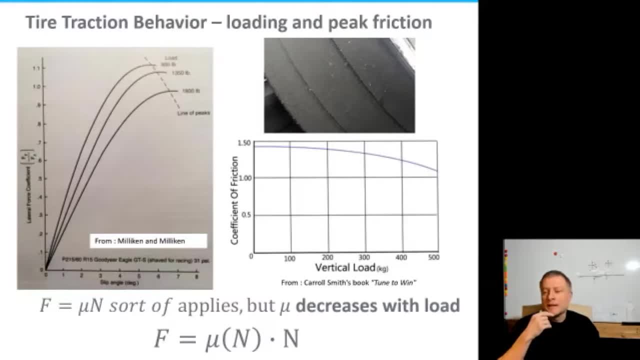 they're poorly understood And I think they remain true to this day. Again, elastic behavior of a tire starts to change into something quite different. as the tire gets heavily loaded, Temperature has an immense effect I'm not even going to talk about today. 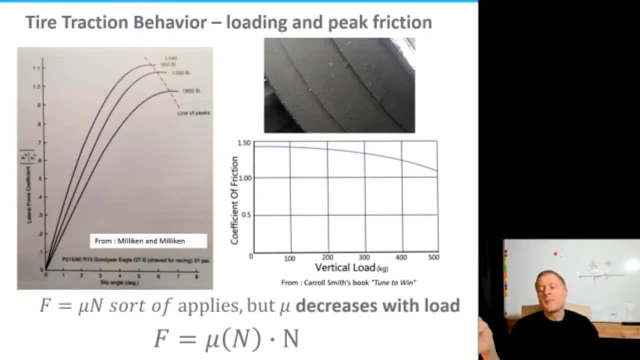 The rubber can melt, it can flow, it can shear And the result is that the frictional coefficient of a tire. it's actually a misnomer. There's no frictional coefficient, There's a force coefficient, as Milliken puts it. because it's not. it costs a number. It varies with the load. 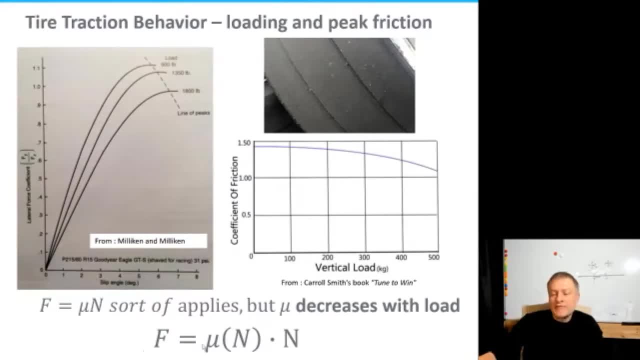 on the tire. So F equals mu, n should really be written as F equals mu as a function of n times n. All right, And as you can see from this graph, the slope of these curves right, which is slip angle versus force, changes with the amount of load. 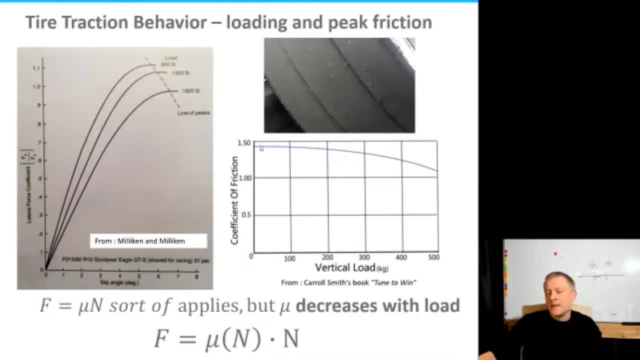 on the tire with the amount of normal force. And so if you were to plot something like the coefficient of friction or the force coefficient as a function of load for a race tire, where it can be, you know, upwards of one and a half. you know of one and a half, it declines relatively. 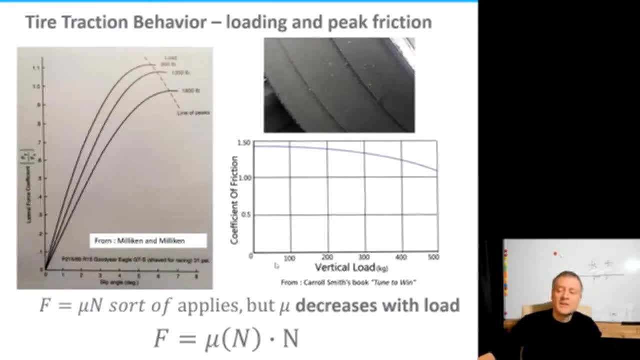 rapidly as you start to increase the load on the tire. Okay, This will vary between tire compounds, different tires and so forth, And also with suspension. I'm not going to get into any of that, but just considering this change in the frictional 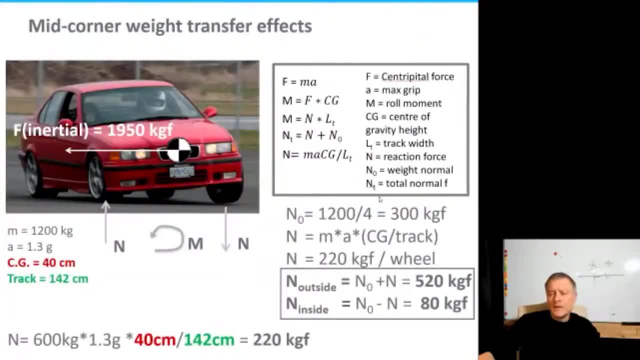 coefficient of the tire, you can sort of see the problems that are going to happen as you go into a turn. Okay, This is, this is my, my daily driver at an autocross course, with my poor daughter in the passenger seat, And you can see what happens, particularly when you mount race tires on a 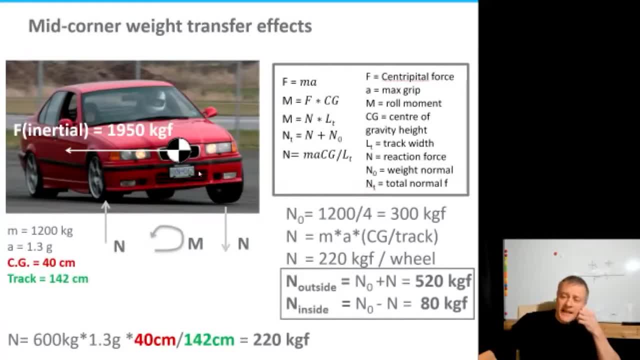 on a road car, You start to get substantial lateral accelerations upwards of 1.3 Gs. And in a heavy, heavy car which you know- and actually this is, this is more like the weight of my race car- 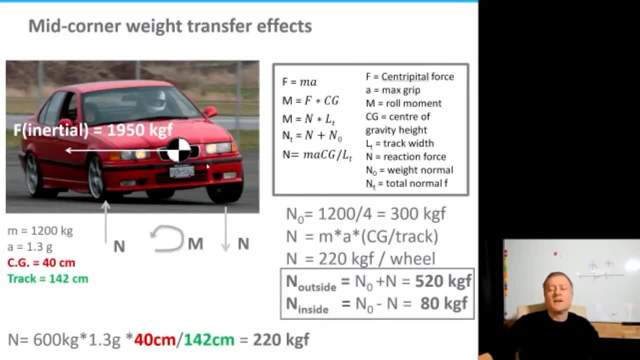 You'll get significant roll moments in the car. Okay, So the center of gravity is relatively high. It's around 40 to 50 centimeters in one of these cars. And yeah, again you know, plotting inertial forces here again instead of accelerations, and apologies to my physics. 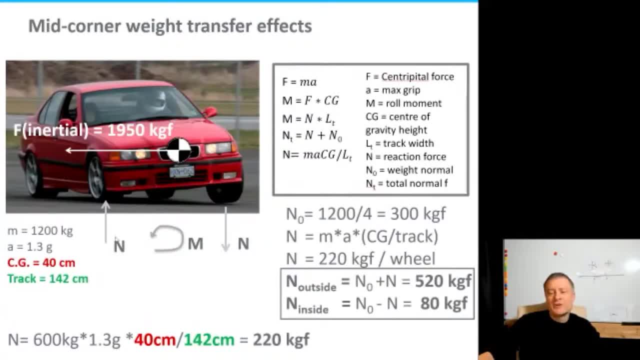 colleagues for that. but effectively you have to counter that inertial force in the turn by a force couple, that's from the outside wheels to the inside wheels, All right, And if you get calculate through that right, I mean the normal force on the tire and not from the 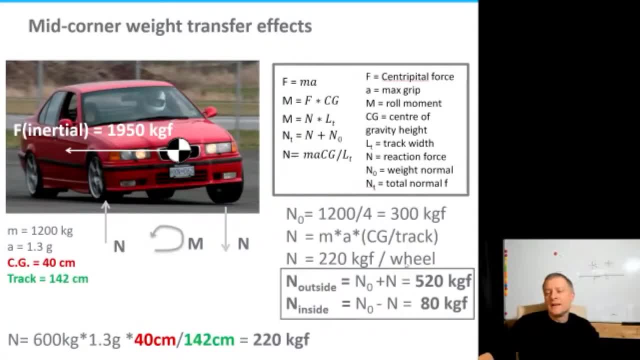 weight of the car is something like 300 kilograms of force per tire. But then there's this moment. that's something like the mass of the car times, the centripetal acceleration of the turn times, the center of gravity, height, and divided by the track width of the car. 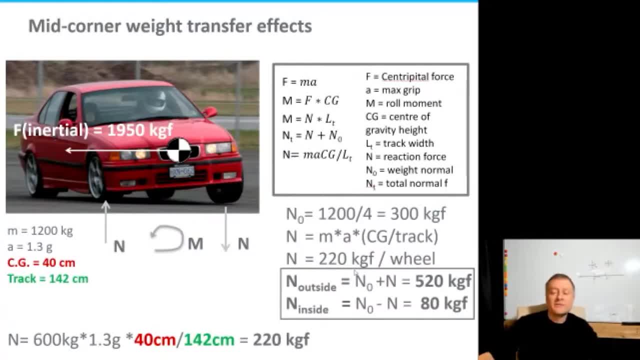 Right, And that can be upwards of 220 kilograms of force per wheel, right. So, as you could actually see in this picture, right, The outside wheels are heavily loaded here They, in this calculation, there'd be around 520 kilograms of force per wheel of normal force, but the inside wheels are almost 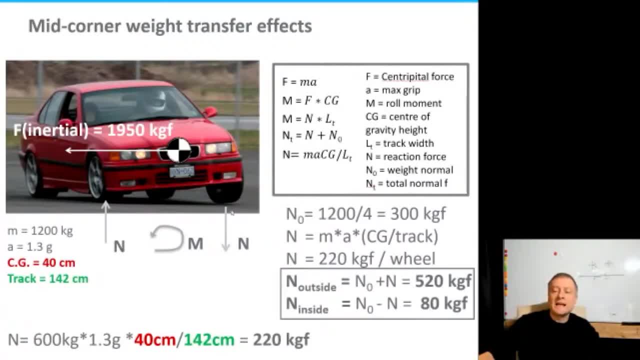 off the ground. They're getting near zero kilograms of force, And I have other pictures of my race car where the front inside wheels is entirely off. It's like a half an inch off the ground, Okay, Where that force has gone to zero. So what does that mean? Right, It means that. 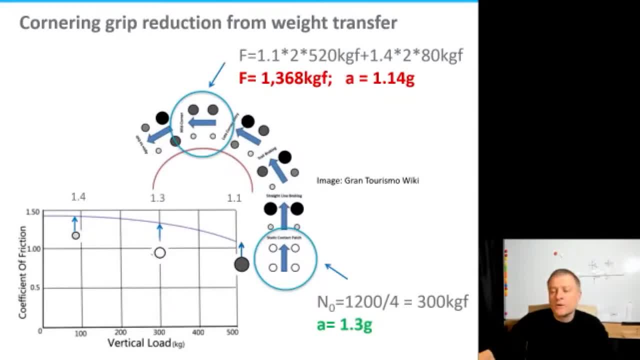 with the car static right, Where it's not cornering, when all the weight of the car is evenly distributed over its wheels. let's say the grip coefficient was such that you could get 1.3 G's of cornering Once you enter a corner, and this is a nice graphic that shows these circles are the width. 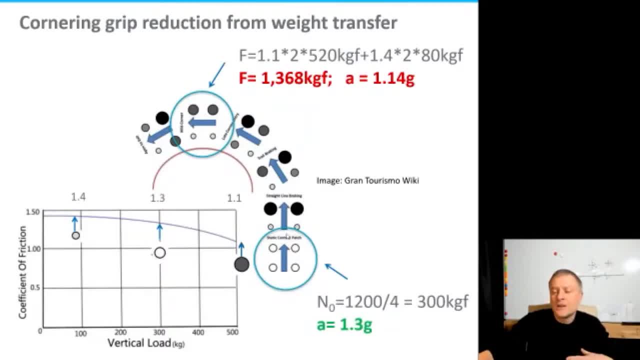 of the circle and the colors related to the normal force in the tire right. So as you hit the brakes, the front tires get heavily loaded from that forward pitching moment And as you start a corner you're loading the outside tires more and more So. looking at the steady state point in the 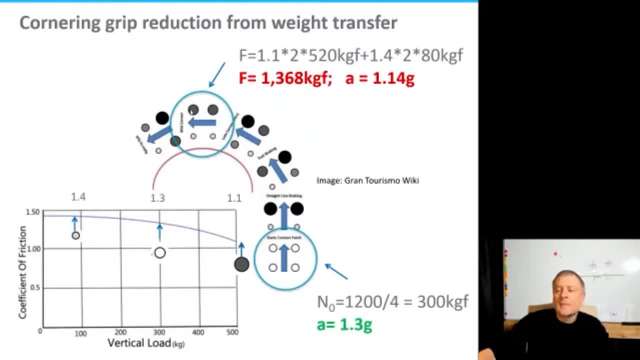 corner where you finished braking and you're not accelerating yet. the outside tires are heavily loaded, The inside tires are not. So what happens on that friction coefficient versus load curve is where your tires are operating- is split. The inside tires are moved up the curve to where 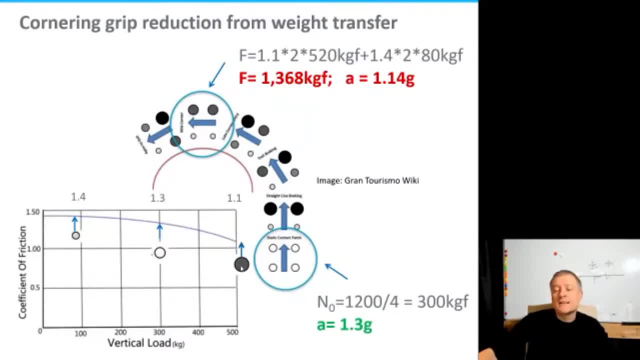 they're getting much better grip, And the outside tires are moved down the curve to where they get much less grip. Now, the problem, though, is that, while the inside tires are behaving more efficiently, the outside tires behaving less efficiently. You think that might average out? 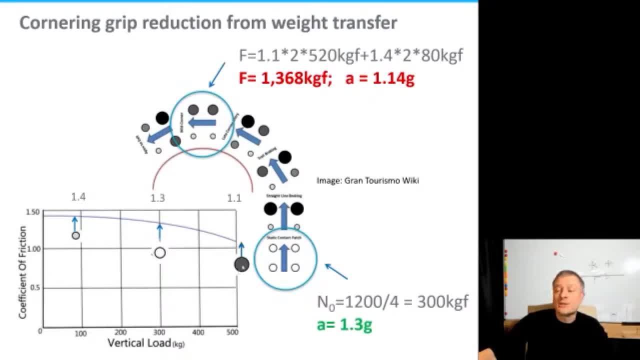 Speaker: 1. And even if the this was a straight line, it still wouldn't average out, because what happens is, of course, the outside tires are carrying more of the normal force and are therefore the dominant source of the frictional centripetal force. So what could have been 1.3 G's of cornering acceleration? 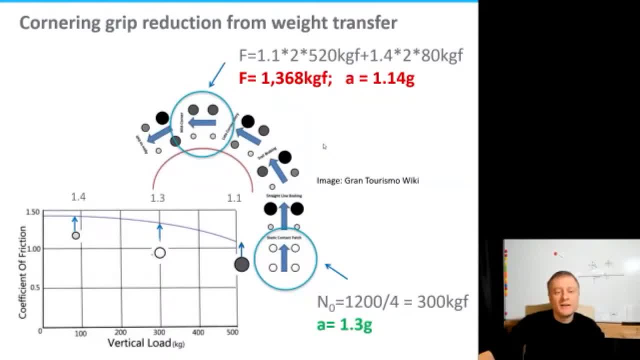 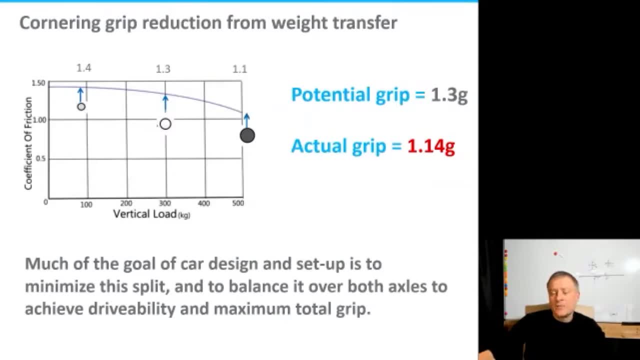 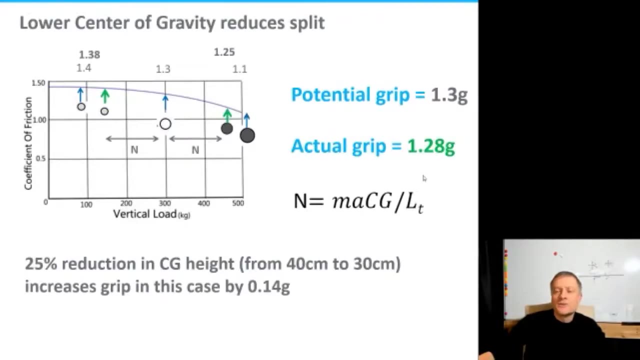 the clients is something like 1.1 G's because of low transfer to the outside tires. So you know, part of what you do in car design and setup is to try to minimize the split And also to try to make it even right. So this is why people lower their cars. 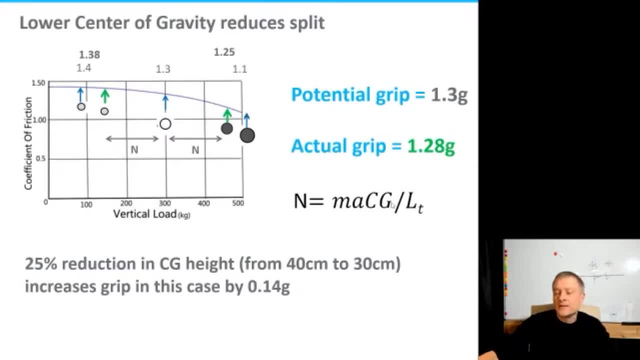 lowering the center of gravity. Remember that raw moment is related to the center gravity over the track width. So a lower center of gravity and a wider car both decrease this effect and actually give you better cornering grip. for, you know, keeping everything else, like your tire compound in tire widths, and all that the same. 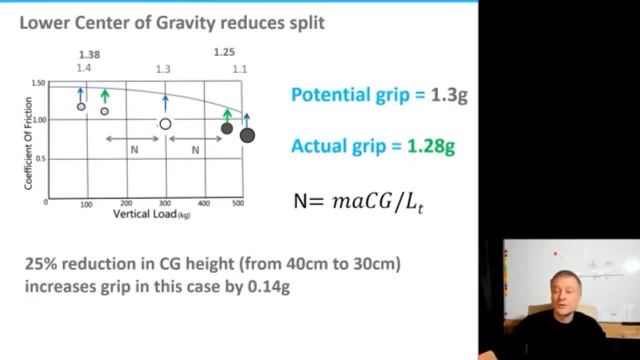 Right. So that's why people lower their cars and that's what you see: race cars being so low to the ground. Um, light in the car has also- uh, you know it feels like it would've were a little lower center component power. But now that you listed race car with the lower center, you're 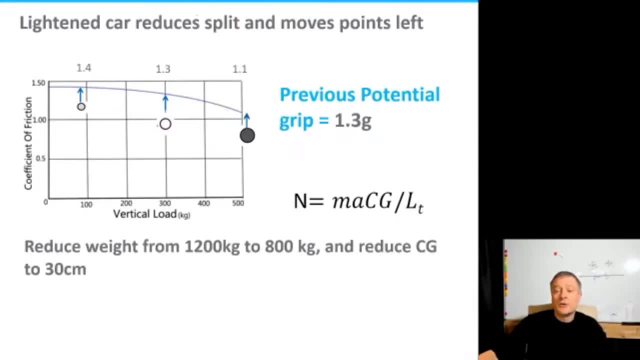 looking at平 difficult, even if the traction in fact would decrease this effect more Een second- to pick big stuff out of that water feature on that. If you look at사� MRS, car automotive is easy to compress. playing on the�� lighten, the car has also an even more dramatic effect, right? Because not only does it reduce, 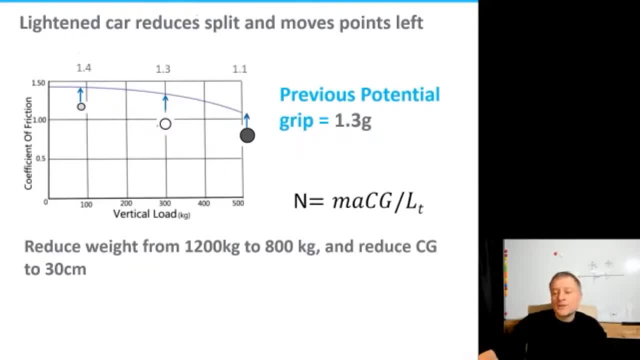 this mass that generates the roll moment, but it also shifts all the points up that curve because the entire car gets lighter right. So you're going from the points being heavily split between the inside and outside tires to being less split but also moved up the curve, And that's why 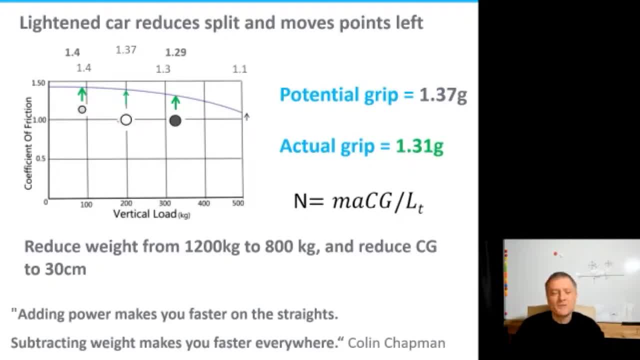 you know, if you talk to someone who's starting in this grassroots racing and asking them, you know. I think everyone thinks the first thing we do to our cars is make the engine bigger or more powerful. And no, most of us do modifications to the suspension, lowering the car and reducing 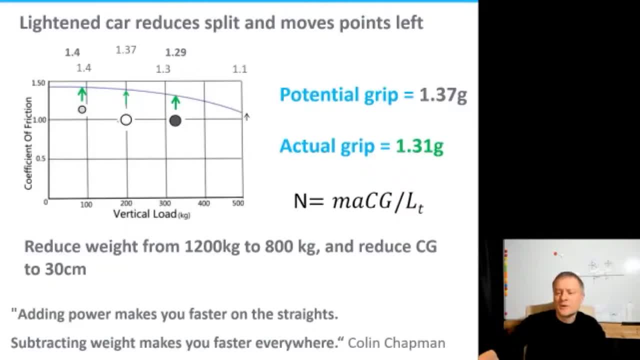 its weight, And then actually the next thing you do is work on your brakes. As Colin Chapman famously said, adding power makes you faster on the straights and subtracting weight makes you faster everywhere. Okay, Obviously you can accelerate faster for a given engine power. 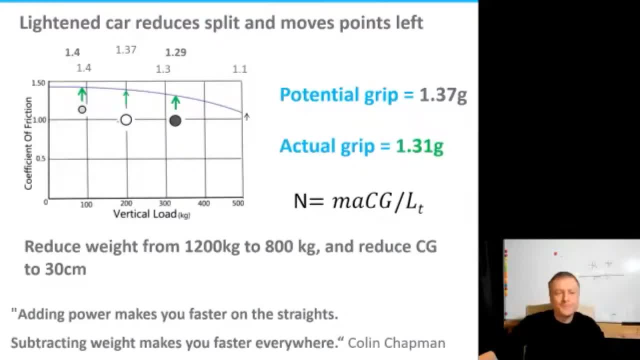 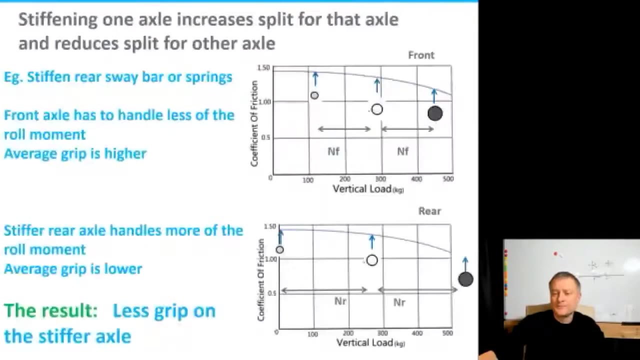 but you get much, much better cornering grip in a lighter car. So that's why I took an angle grinder to my BMW and chopped off more panels than you want to know and replace them with styrofoam and carbon fiber, just to try to reduce weight wherever I could. Now the other challenge, and this is one. 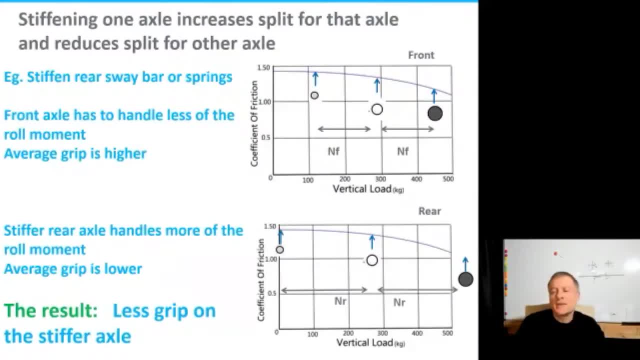 of the challenges of a race engineer is making sure that that weight split happens evenly, or at least in a way to maximize utilization of all the tires right, Partly to make sure that the car is drivable. So you want to make sure that, as you. 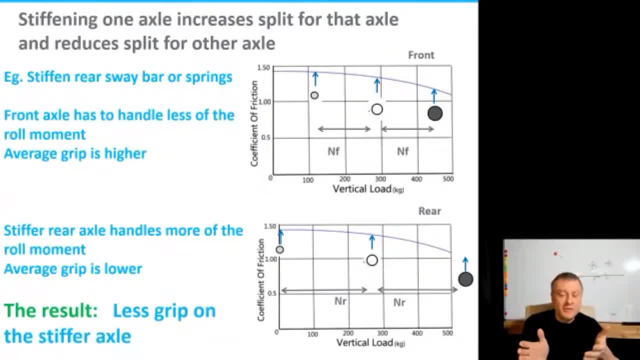 In the middle of a turn that the front axle is not slipping more than the rear axle right, Or vice versa. So you don't want a lot of understeer or oversteer in the middle of the turn And when you do that the way you do that, if you think of the car really it's relatively rigid body. 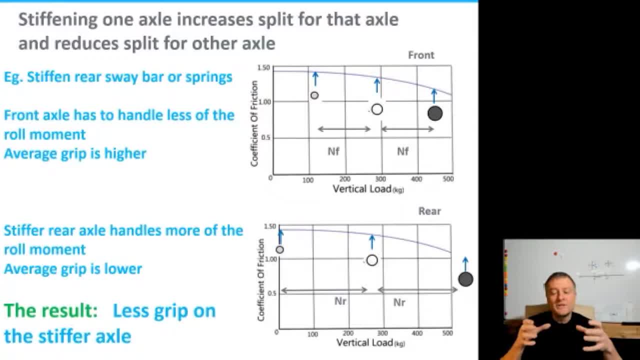 right. So as it tries to roll, you've got to ask which of the two axles is going to counteract that roll moment. It doesn't necessarily have to be the same on both axles. So a thing we commonly do is adjust the stiffness of our front suspension or rear suspension by changing the steering wheel. 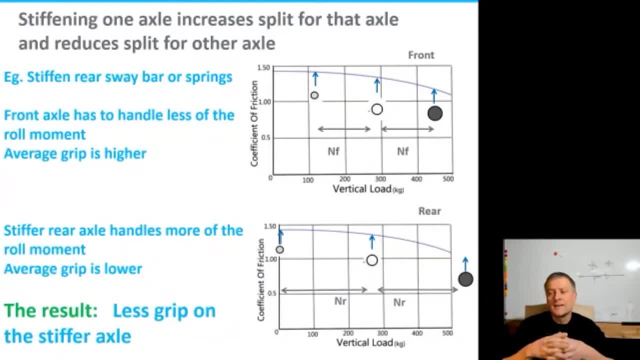 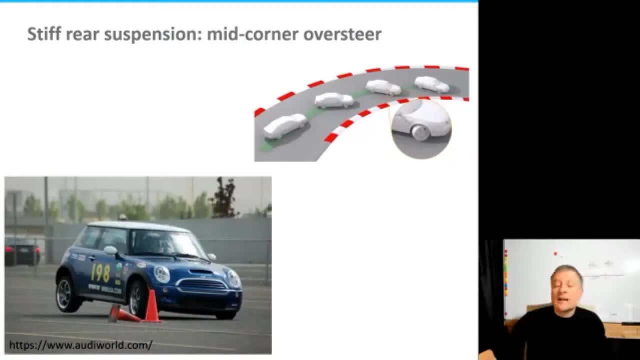 Springs are what's called the sway bar to balance the effect to which each axle takes the roll moment. So if you want a car to rotate well into a turn, you would actually make for a very stiff rear axle, right. So here's the rear axle, here's the front. If you stiffen the rear axle more of 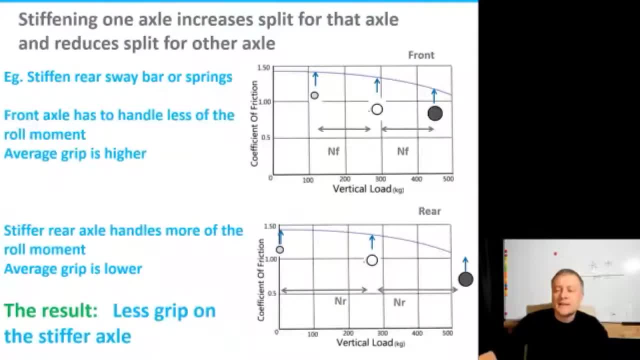 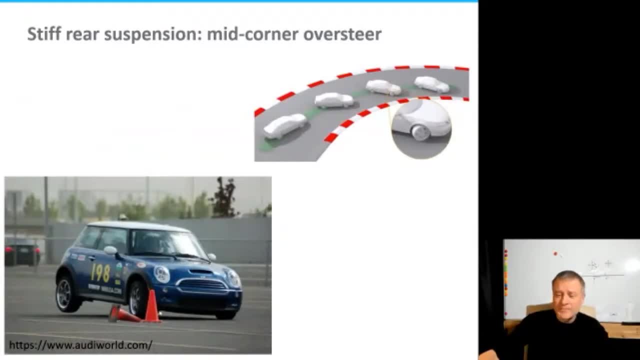 that roll moment is taken by the rear wheels less by the front, And you get situations like this where in fact, the car will lift its rear wheels going around a turn, And that can make for, if you overdo it, it can make for dramatic behavior. 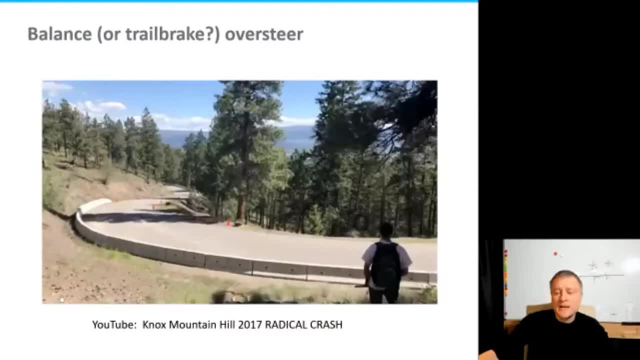 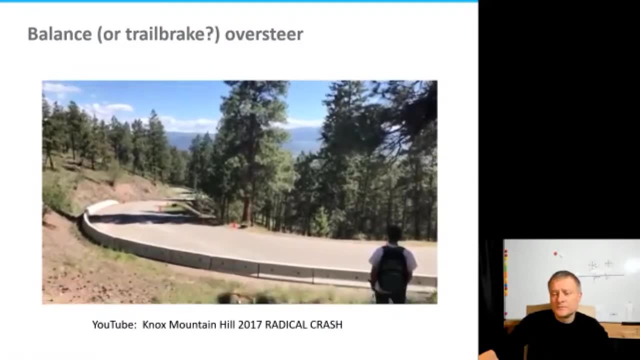 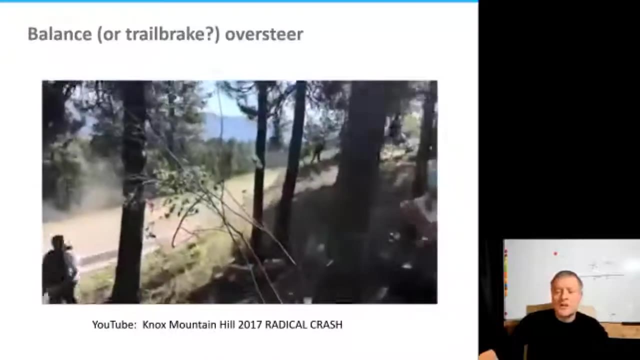 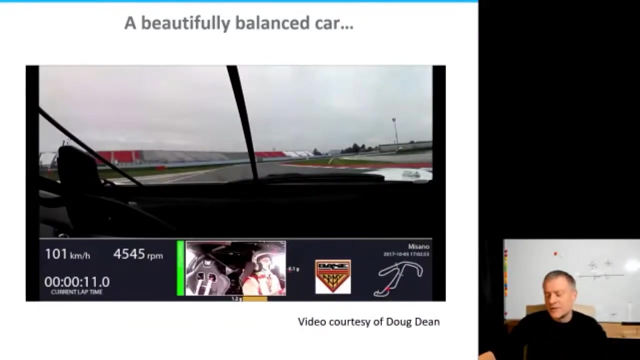 Here's another one of my fellow competitors at Knox Mountain with a car that was a little bit prone to oversteer. So as you saw the car come into that turn, the rear axle lost grip long before the front and got the rotation. He was fine, of course, As I think I saw someone saying: 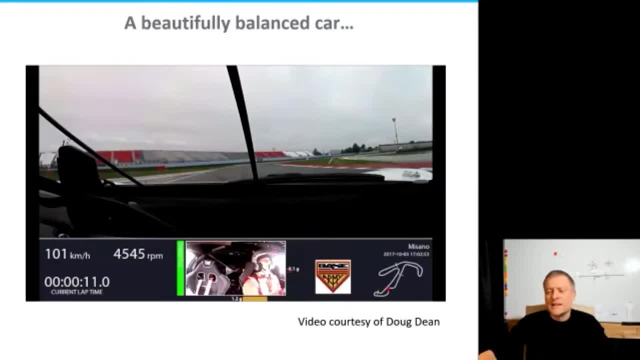 in the chat we are. I can tell you later about how we're protected, but we're, yeah, there's a lot of protection around us as drivers, keeping us safe in crashes. So you know, ideally, if you get those things, 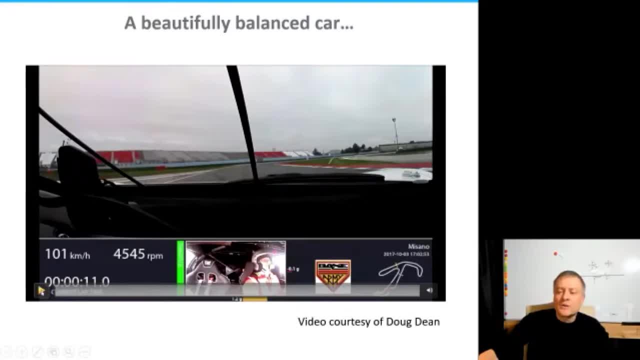 balanced right. you can set up a race car to where you're going around corners at incredible speeds with your tires effectively sliding, And you can hear in this video the screech of the tires in the background and the car staying so steady that in this case, it was incredibly easy. 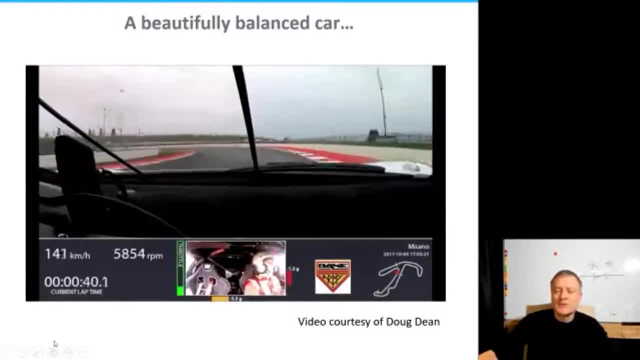 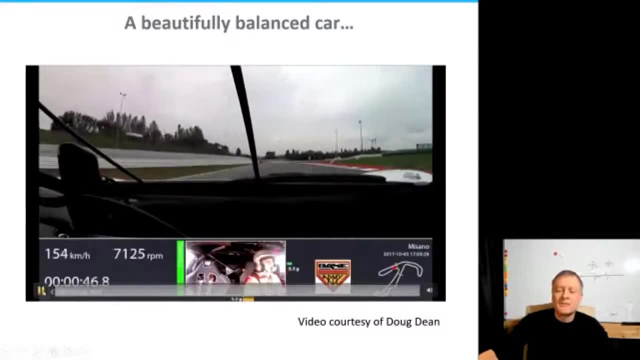 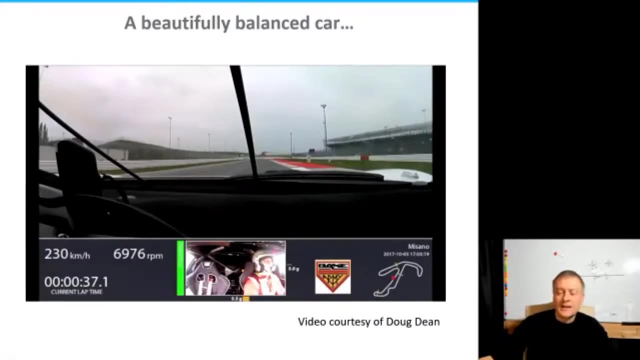 to drive Coming into turns at 200 kilometers an hour. Yeah, you can barely make out the tires- the tires starting to complain. But I can tell you that it was so relaxed in that car- because this is the 488 Challenge and that day was particularly well balanced- It was just an absolute pleasure to drive. 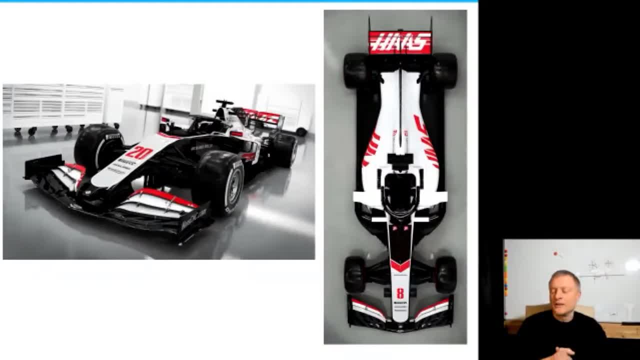 So that's. you know that's such a brief glimpse. I, you know I'm trying to squeeze what's a three hour talk into 50 minutes. The reality of race cars now, particularly the Formula One cars, is that while they have to deal, 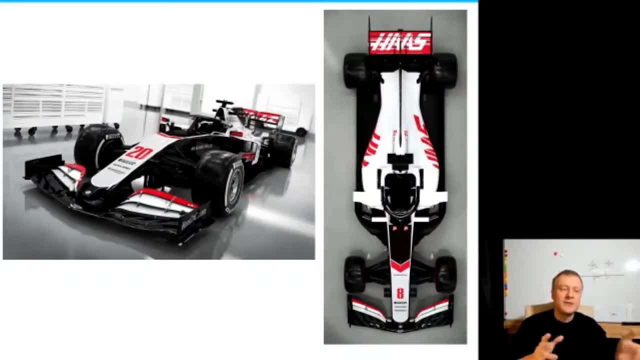 with all those mechanical trade-offs in design, and what I've given you is about 1% of what they really have to do. You know, the speeds are such that aerodynamics play an absolutely dominant role. So, on top of all the mechanical grip that they have to try to optimize, they also have to 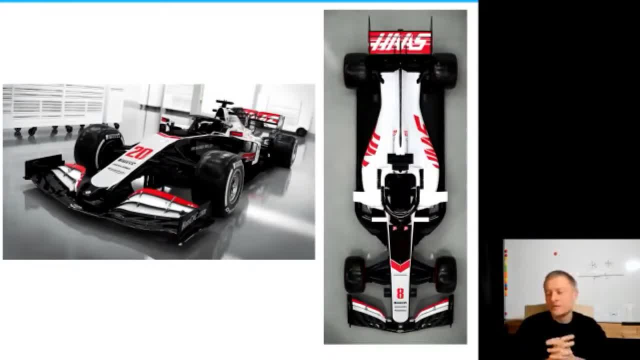 optimize aerodynamic balance and reduce drag and so forth. So hopefully that gives you a bit of a appreciation for both The car driving and the car development. And you know, hopefully with that increased appreciation I will let you enjoy my last video and one little clip from you know, being Canadian, obviously a famous battle between 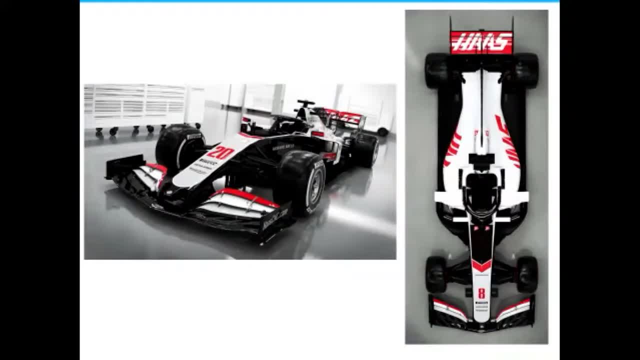 Gilles Villeneuve, one of our most famous Canadian Formula One drivers, and Rene Arnaud at the 1979 French Grand Prix. And just watch the skill of these drivers as they're operating at the limit of grip inches from each other and actually occasionally touching the ground. 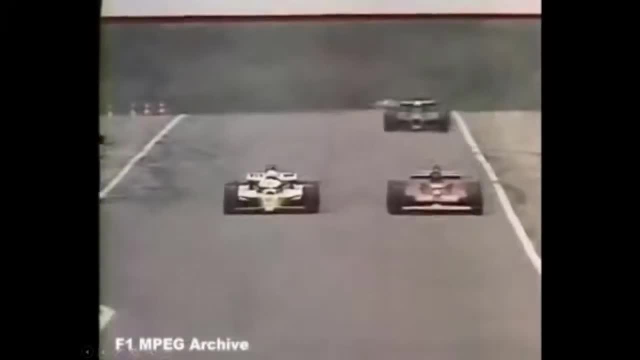 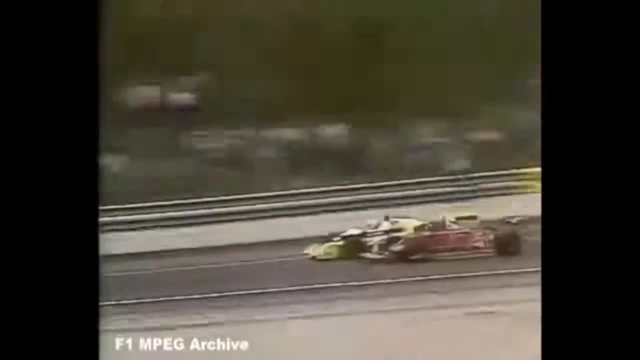 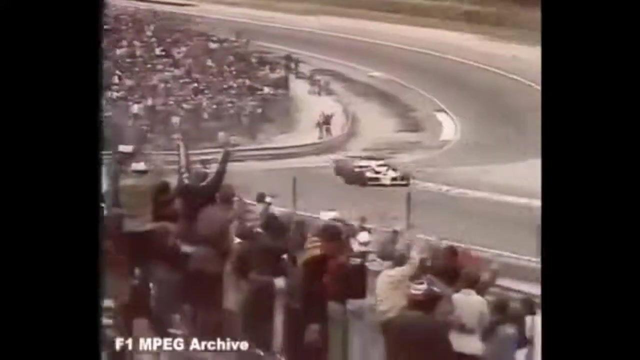 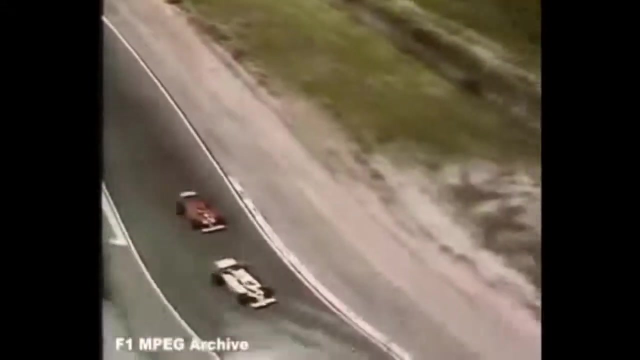 And it's there that they can pass, and Arnaud's going to do it. Rene, Arnaud is challenging for second as they come up to Villeneuve, but Villeneuve will not give way. Arnaud's got the inside line and the shorter line And he takes second place as they go into the right-hander on the left at Sainte-Liaire. And now Rene's indeed our first and second in the French Grand Prix, And the French crowd is going mad, roaring in the background. 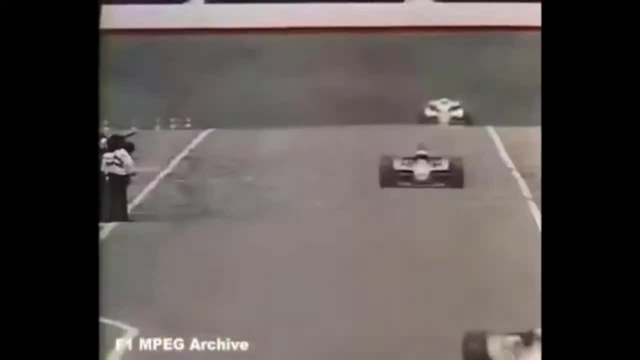 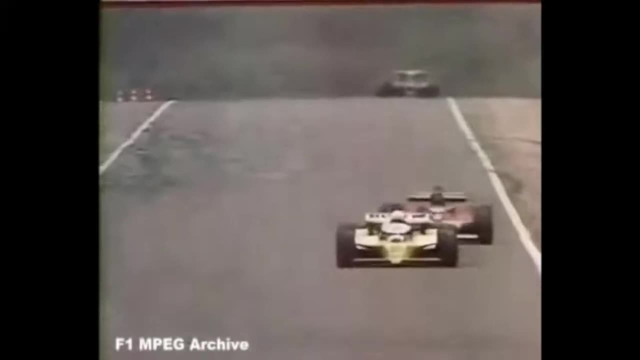 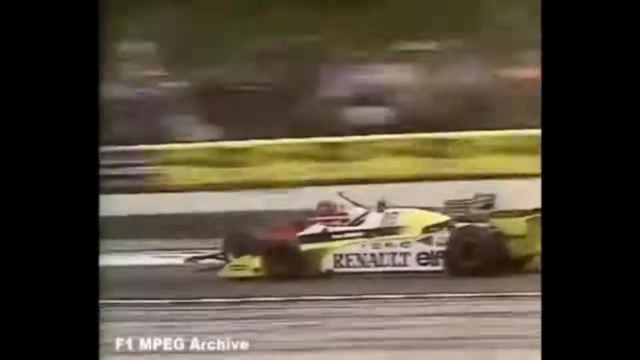 This is incredible. The twin turbo Renaults appeared at Monaco, not their circuit, And now we're into the start of the 79th and last lap of one, with Rene Arnaud second and Villeneuve done it. Incredible. Villeneuve stood on everything locked up his tires, got the line and he's back into second position on the last lap of one. 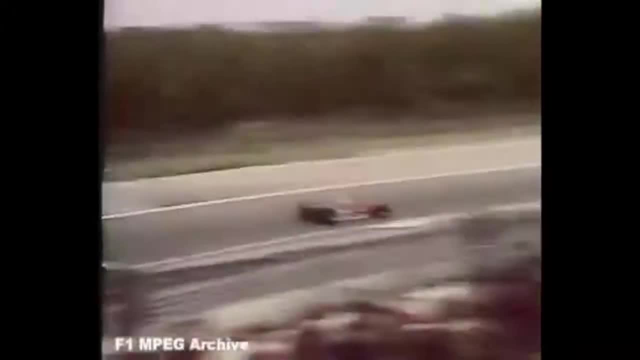 And the French crowd aren't very happy about that, and who can blame them? This is incredible. This is the 79th lap in this 80 lap historic French Grand Prix. This is incredibly exciting. This is incredible. This is the 79th lap in this 80-lap historic French Grand Prix. 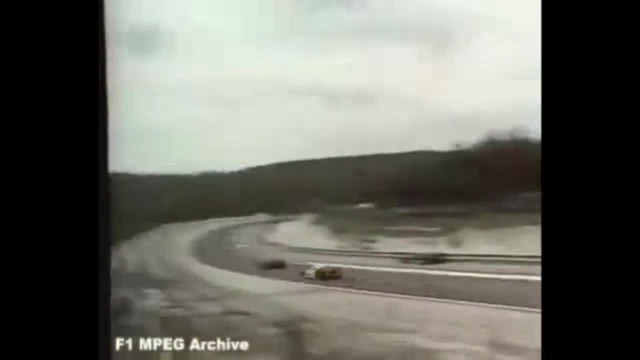 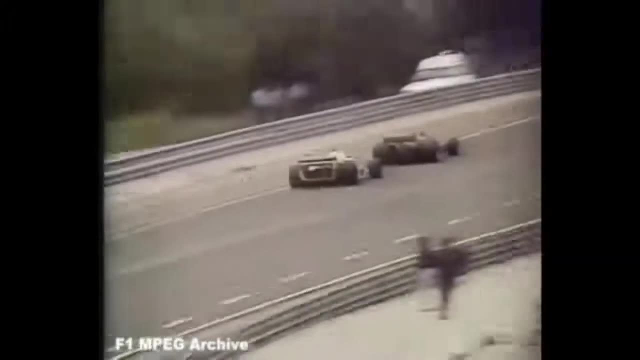 Grand Prix, the oldest Grand Prix of them all. This is the 65th Grand Prix and there has never been a more exciting battle for a major position than this one, with such French interest. Jambouy still ahead And he's close right up on Villeneuve and he's going to try. 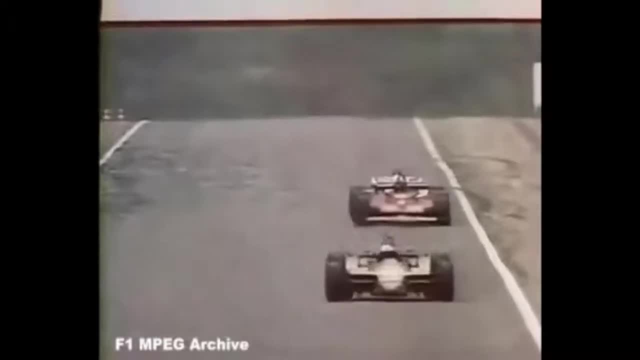 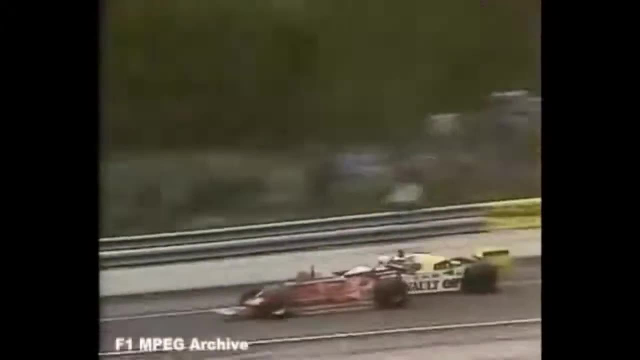 again. They're coming into the start of the last lap behind Jochen Maas in the A2 Arrows And Arnoux does it, does he? And Villeneuve knocks up And Villeneuve has had to go wide and Arnoux is on the inside as they go round Villeroi, He's got the shorter line, He's.